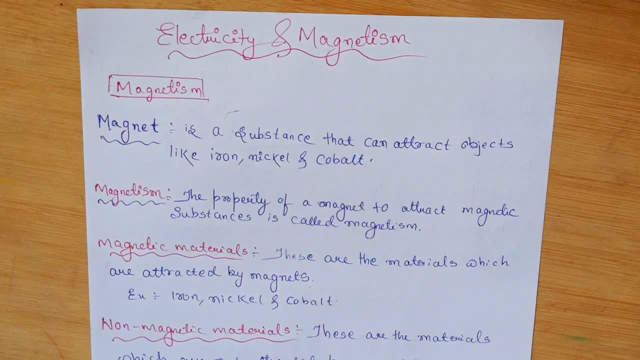 So a simple answer to that is that a magnet is a substance which can attract other substances. Now, other substances can attract other substances. What kind of substances are there in other substances? That is important. A magnet cannot attract everything. A magnet basically attracts what kind of substance? 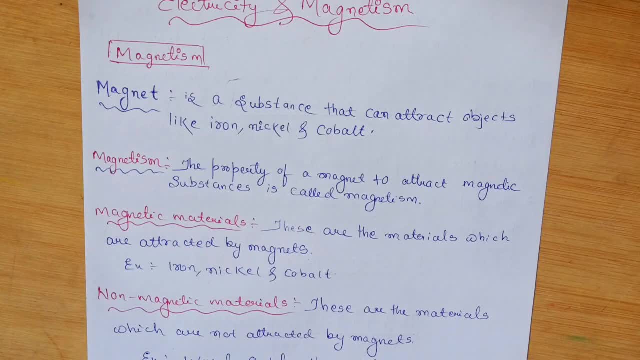 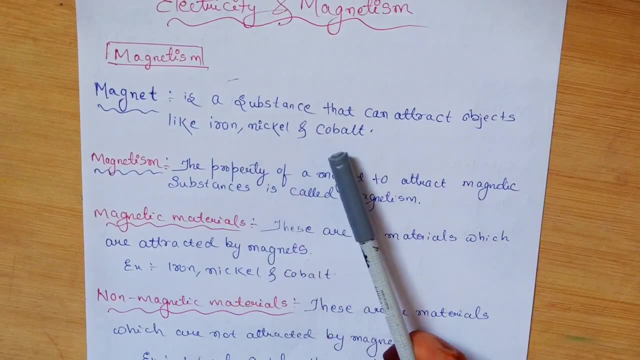 A magnetic substance, And we can say that a magnet attracts magnetic materials towards itself. So here, kids, look, there are some substances' names Like iron, nickel- what is nickel in Hindi, I don't know- And cobalt- what is it called? I have no idea. 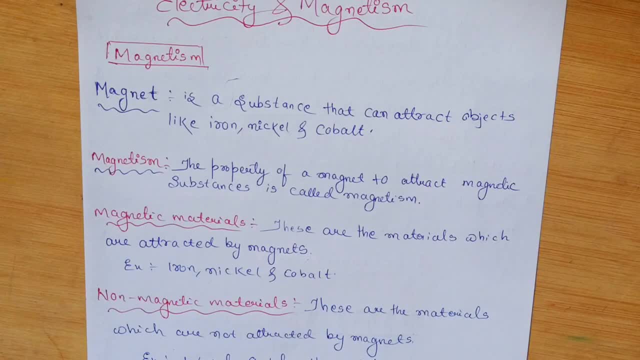 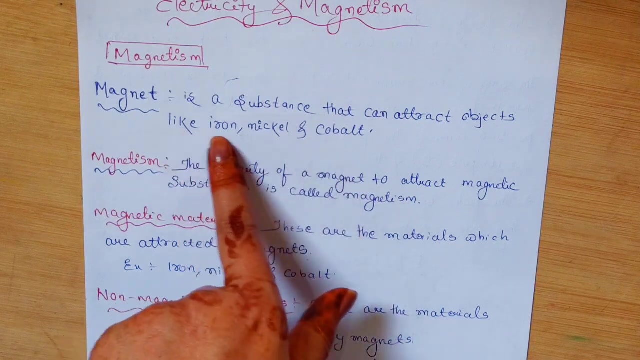 Normally it is used worse by calling it nickel and cobalt. Okay, so a magnet is a substance which attracts magnetic materials or magnetic substances. Like what kind of magnetic substances? Like iron, nickel, cobalt. These three names are very important. 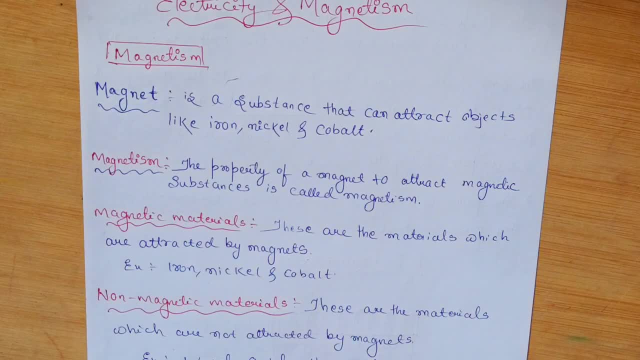 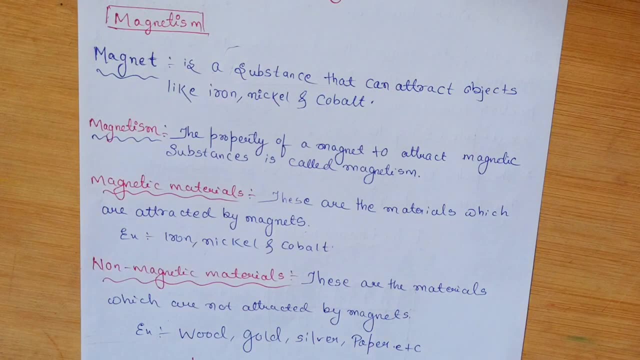 You must remember this. Then, second one is magnetism. See, magnetism is related to magnets. So what is magnetism? So, magnetism means it is a property of a magnet. It is a property of a magnet. What is the property of a magnet? kids? 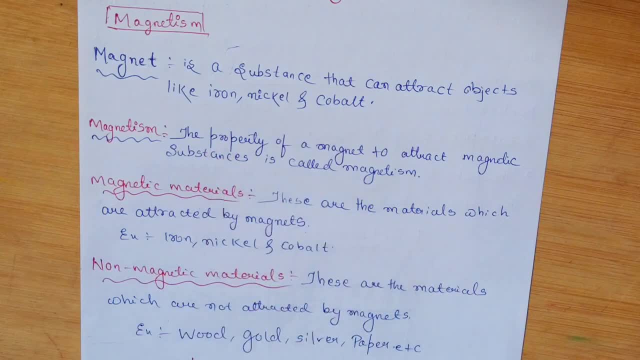 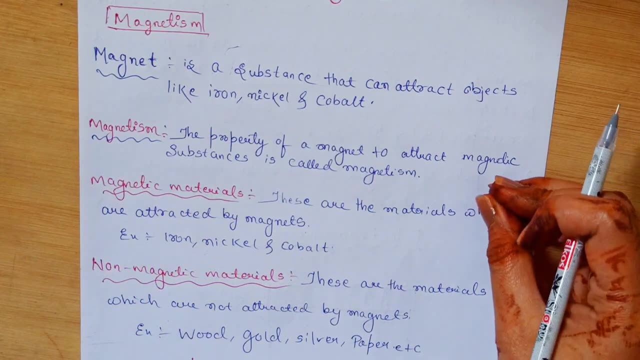 To attract magnetic substance towards itself. So the property of a magnet is the one which attracts magnetic substance towards itself. Like, if you bring a magnet, then what will a magnet do? If you keep a pin here or any iron material, what will a magnet do? 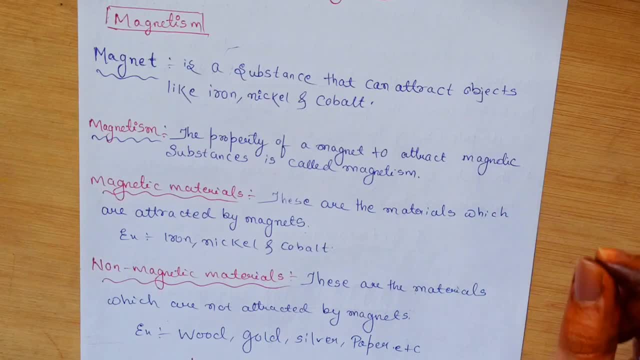 It will attract it towards itself. It will attract it towards itself. So this property is called magnetism. So magnetism is not a thing, it is a property. Whose property is it? It is a property of a magnet. 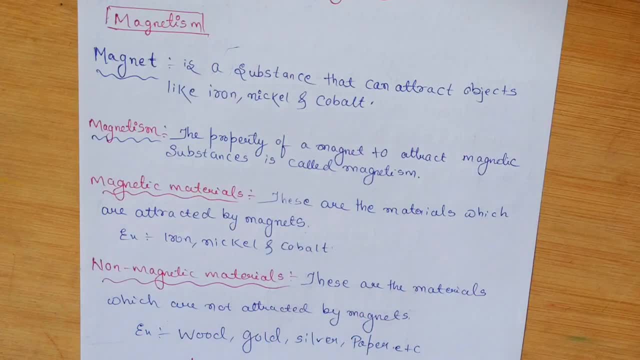 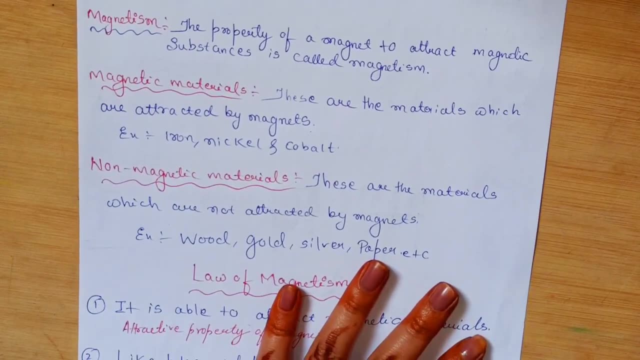 What property does it have To attract magnetic substances? What types of magnetic substances have there, Like iron, nickel and cobalt Now- magnetic materials or magnetic substances? So what are magnetic materials? Magnetic materials are the materials which are attracted by magnets. 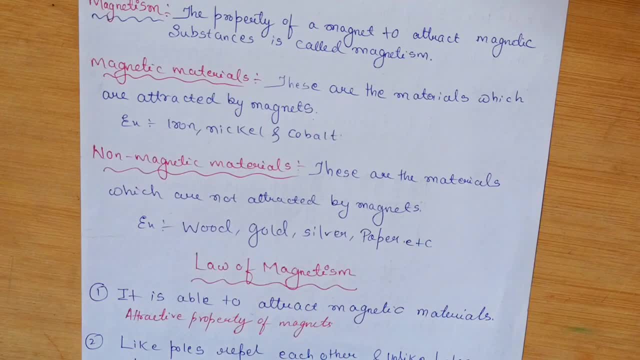 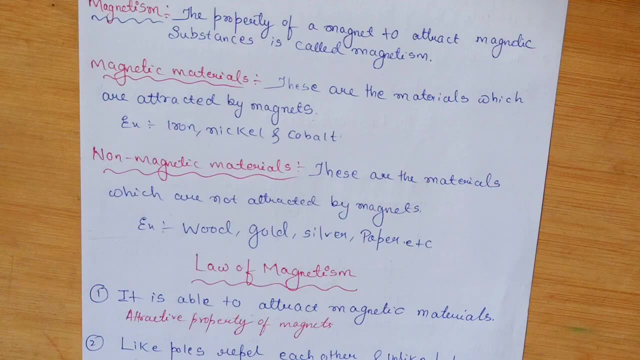 Means magnetic materials like iron, nickel, cobalt. These are the substances which are attracted or which gets attracted towards a magnet. Example is also visible here. you must be able to see the same way, see the same way, as I told you already that 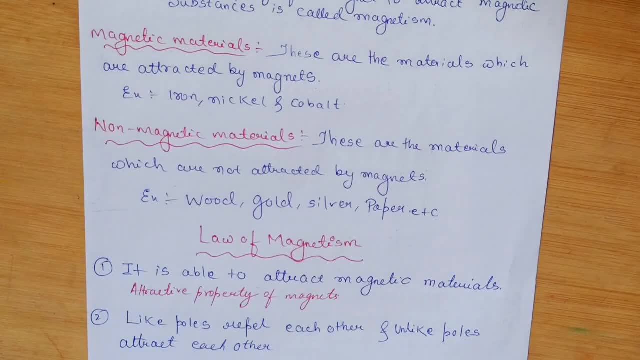 every substance can't be attracted by the magnet. okay, the one who will attract- we call it magnetic substance or materials. okay, but if I talk about this pen, will this pen be able to attract the magnet? not at all. this paper also not be able to. this wooden. 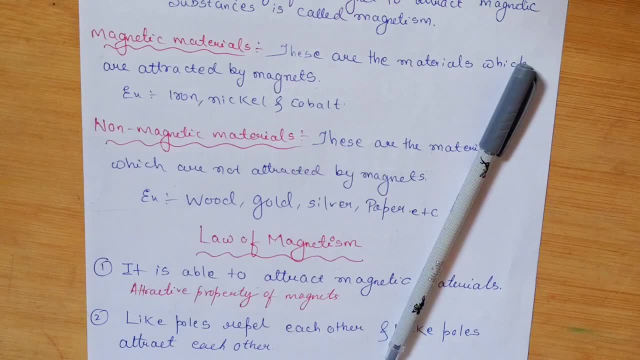 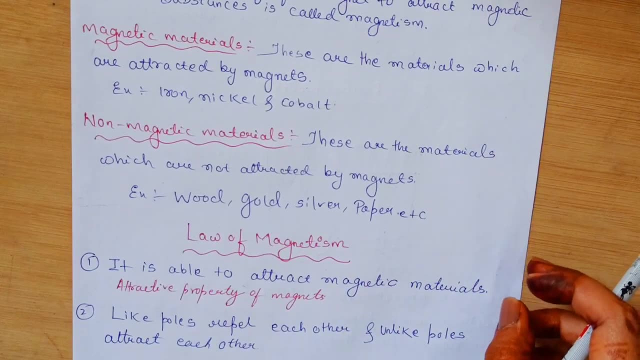 paper also not be able to attract the magnet, so we call it non-magnetic materials. so non-magnetic materials, basically those materials, those substances, those things which are not attracted by magnets, which are not attracted by magnets- for example, there is wood paper. 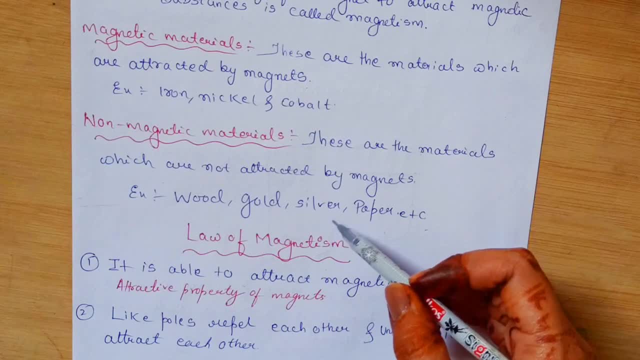 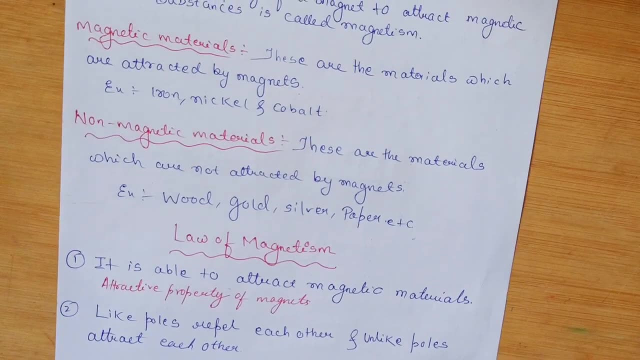 you can write plastic, you can write pen, gold, silver, etc. etc. so this was the basic concept on the magnet. now we will read certain laws of magnetism. okay, now we will read laws of- let's do laws- laws of magnetism. 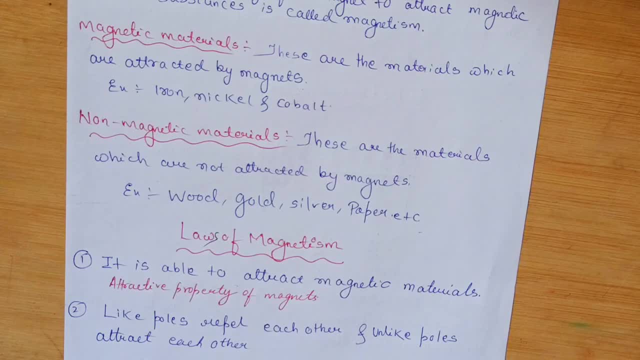 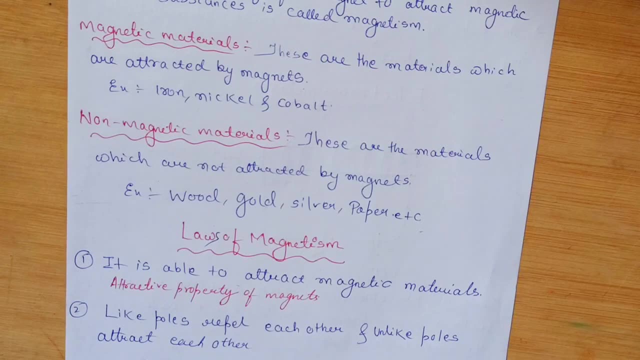 now, what is the law of magnetism means? here also, you will read things related to the properties of magnet. the first property- see, kids, this is above the magnet. this is the property of magnet. the first property of magnet, that is, it is able to attract magnetic material. 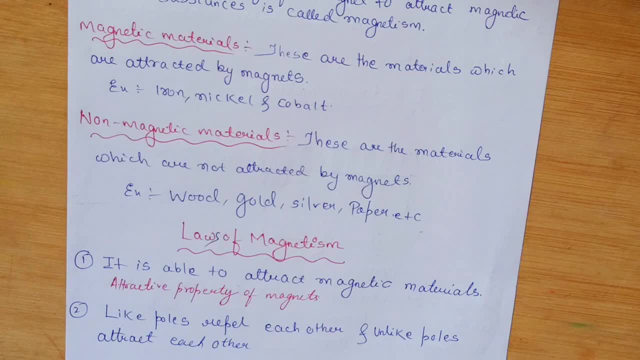 here it is for magnet. okay, so the magnet is able to attract magnetic material. definitely, we have read that the magnet can attract iron and nickel, so we have written here that it is able to attract magnetic materials. so this line shows the attractive property of 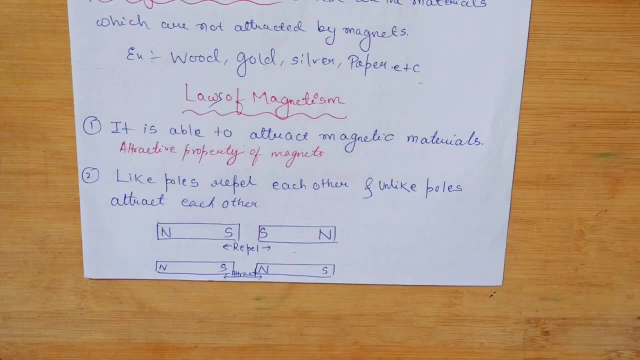 magnets: attractive property of magnets. now the second property is very easy. you have already read in classics. second one is about repulsion and attraction. see about repulsion and attraction. it is very simple. now here you will see two diagrams. this is the first. 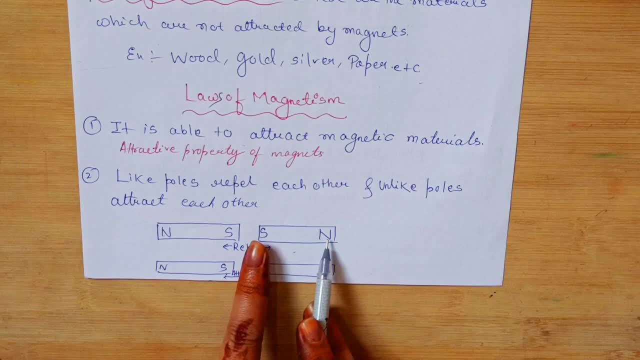 second: okay, this is one magnet, bar magnet, and this is the second magnet. okay, two bar magnets. we have taken here what we have done. now see here the poles you are seeing S and N. we will discuss about this in the next next, in the next point, but I will still. 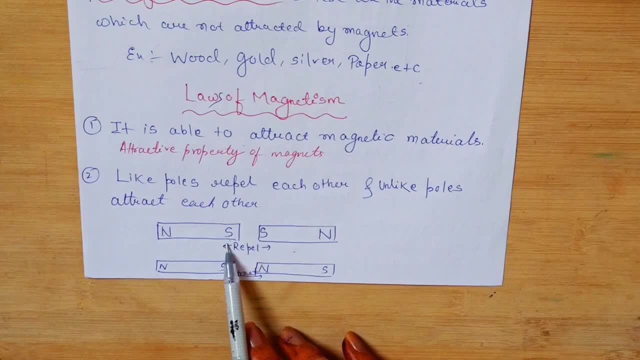 tell you that any magnet you take, it has two poles. one is north, one is south. so I have made it north and south according to me. okay, so I have taken two bar magnets here and the second time we have taken both the bar magnets close to each other, that. 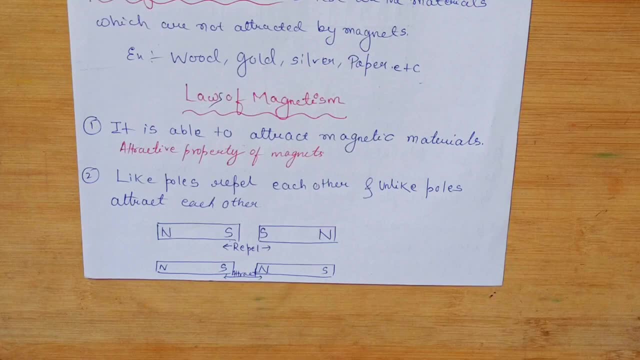 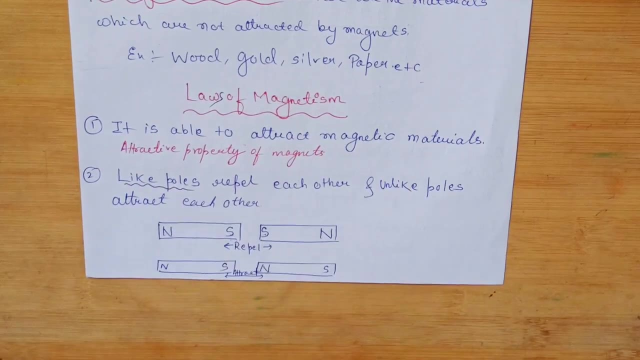 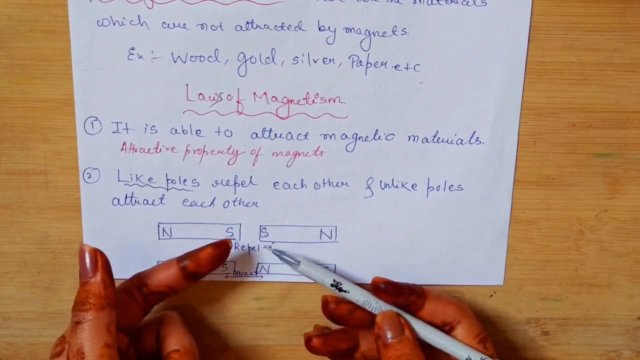 is we have brought them near and how do we arrange them here? it has been arranged so that two, which is like poles, like poles, means same same, same, same same. so see here: S and S means two south poles, two poles of different magnets. when I brought them 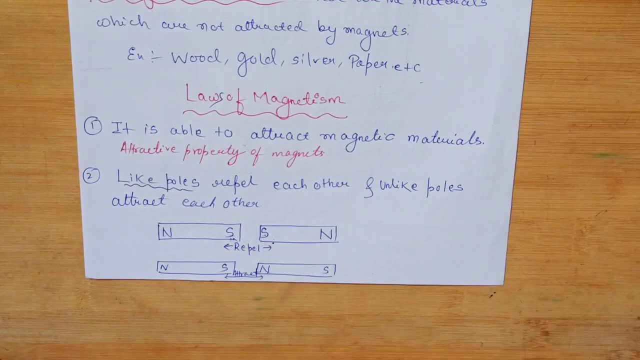 near. so we have observed there that they repel each other. they push each other away means like they push each other away. okay. and the other magnet we have brought them, unlike poles. when will you see? unlike from here? I am writing here like poles so that you will not get confused. 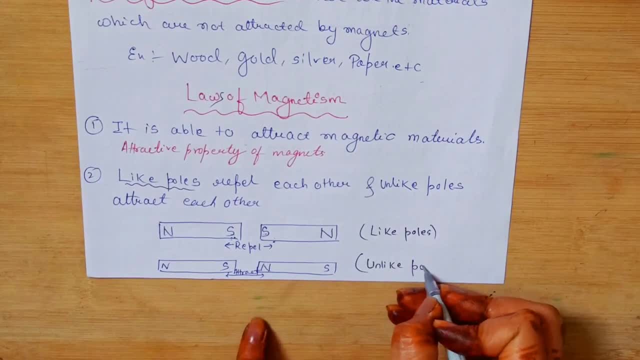 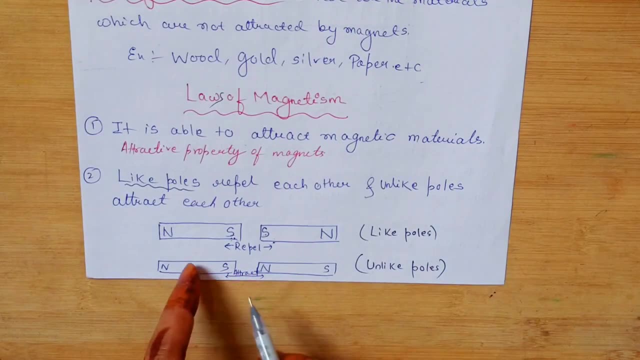 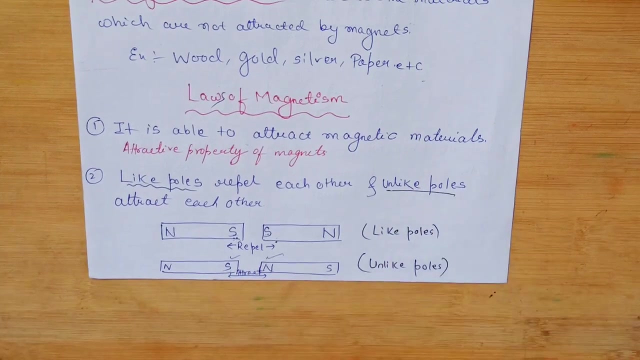 and here it is about unlike poles. in this case you can see that here two different poles are brought close to each other. here are two different poles, like here is south pole and here is north pole, so for different poles we use word unlike poles. so when we will bring unlike poles close to each other, then we will get to see attraction. 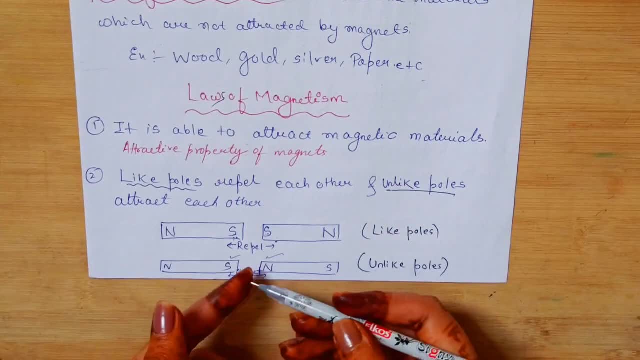 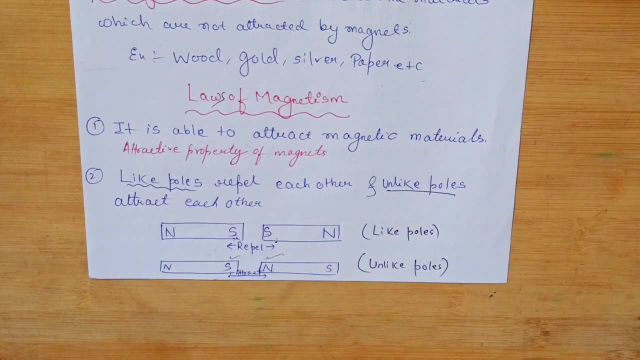 means we will see that these two magnets are attracting each other. they have come close, but in the first case they were running away from each other, they were repelling each other. obviously opposite attracts. so here opposite is attracting and the same is repelling each other. 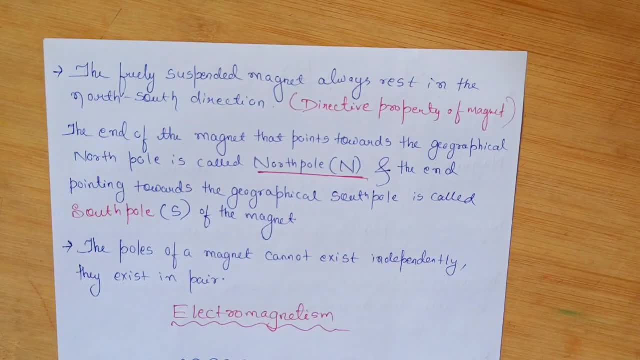 now, the next law of magnetism is related with directive property means it is related to direction. so now if we take a magnet- as we have taken a magnet once- and kids will tie it with a thread and will align it and will suspend it freely, means they will tie with a rope. and if you will hold the rope and will leave magnet, 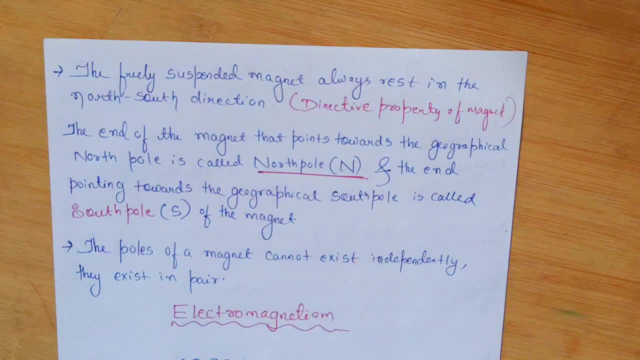 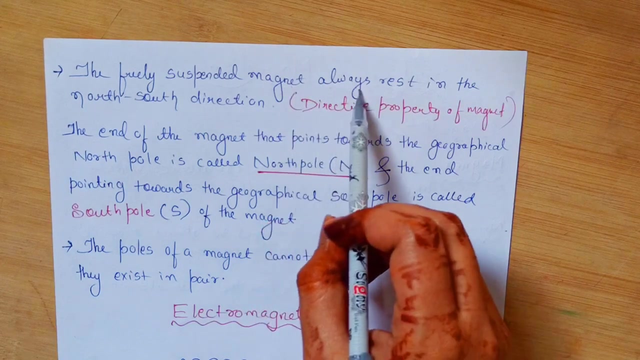 magnet is moving downwards like this, we will see that in some time the magnet will align itself in a particular position, in a particular direction, and that direction is north and south direction. it happens so. So the freely suspended magnet always rests in the north-south direction. 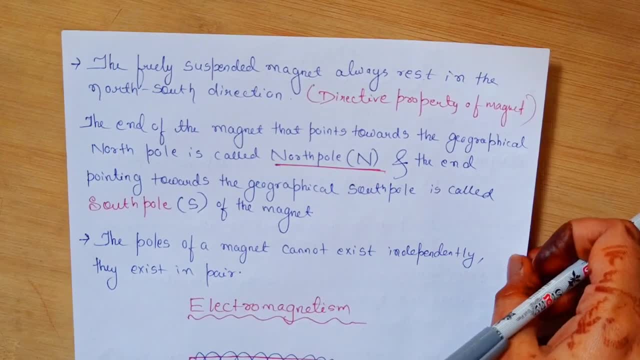 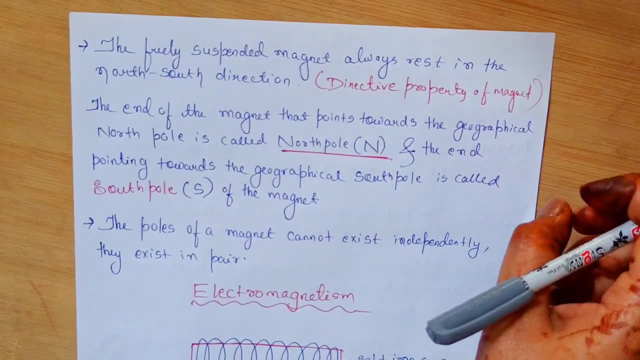 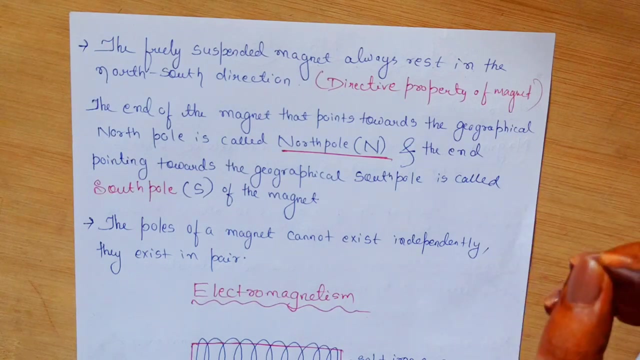 This happens. You will know this by experimenting. You will know this by experimenting The freely suspended magnet. if we take any freely suspended magnet, then it will always align towards the north and south direction. If you want, you can do this at home and see. 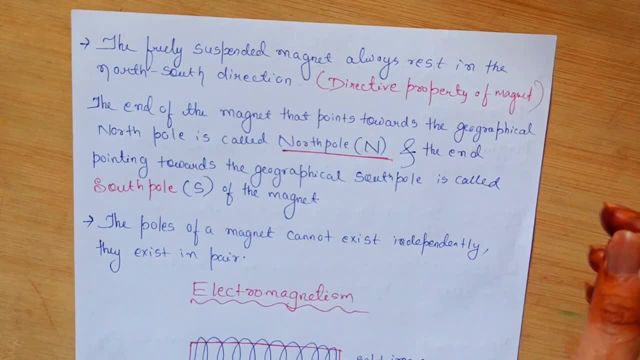 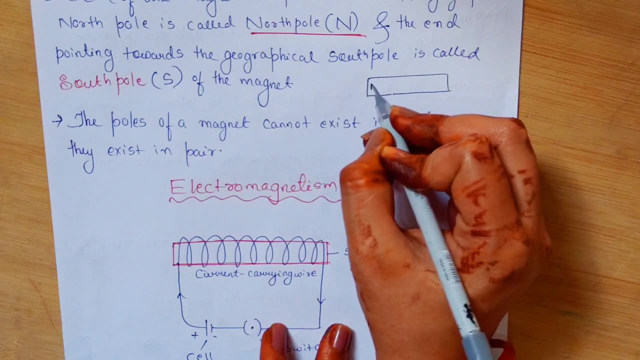 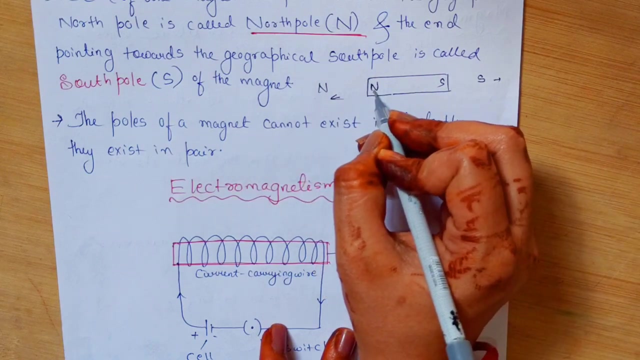 So this property is called the directive property of a magnet. Now here, if this is a magnet and the magnet is in the north-south direction, suppose this is the north direction and this is the south direction. So the pole of the magnet which is normally in the north direction, 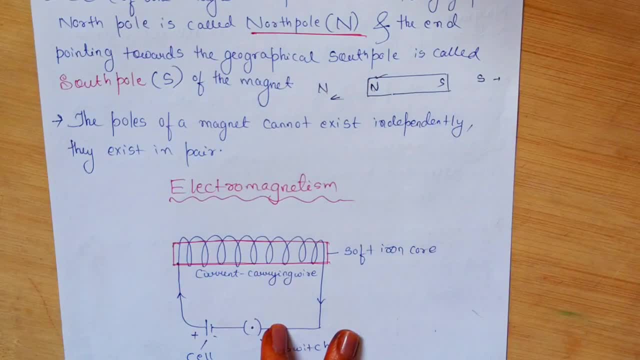 we will call it the north pole, And the pole of the magnet which is aligned towards the south direction, we will call it the south pole. So these are the poles which are designated. One more thing, One more thing which is very important, very important children, very important point. 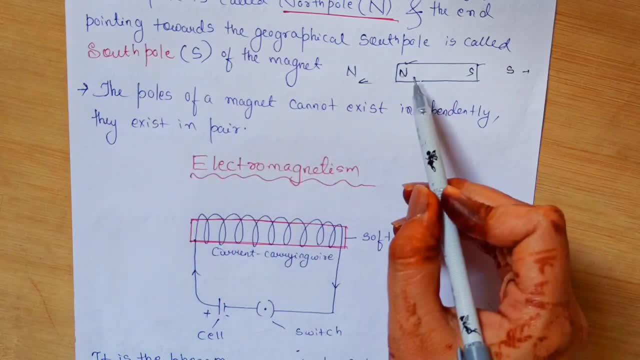 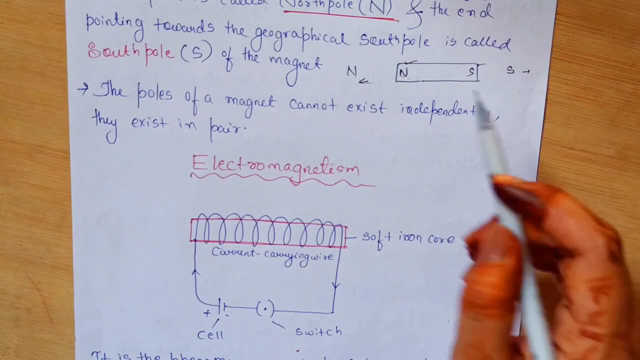 Poles of a magnet always exist in pair. The poles of a magnet like north pole and south pole. If anyone uses the word poles of a magnet in front of you, then there is a discussion of both north and south. So the poles of a magnet, they always remain in pair. 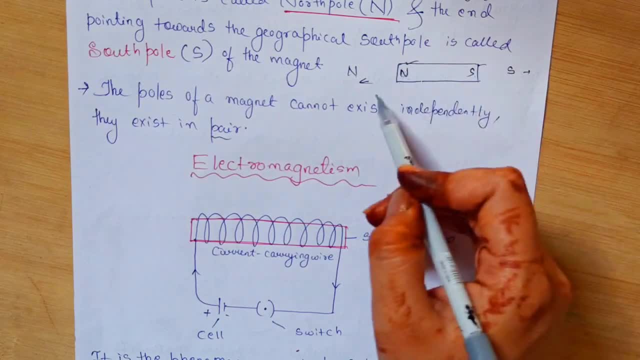 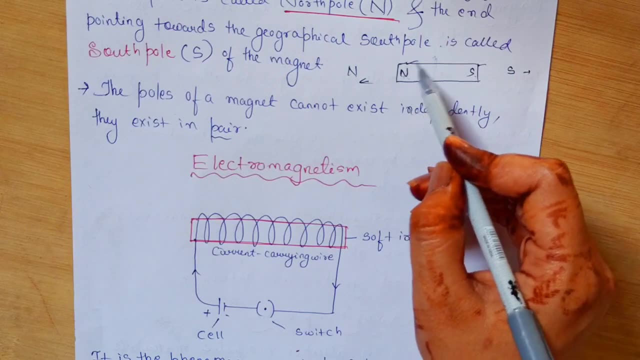 They never remain separate. Okay, Like here. look, both are present in this magnet. There is north and south. If I break the magnet from here, from the middle, then here the south will come. It will not happen that if I break it. 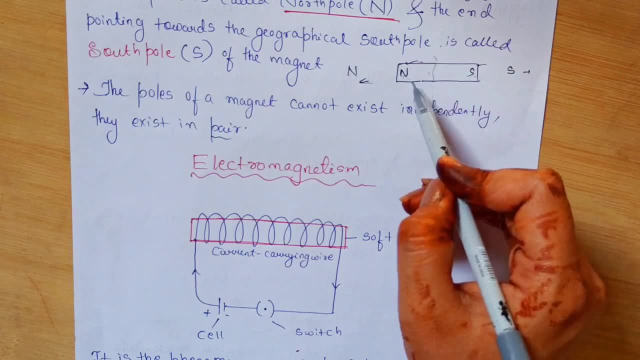 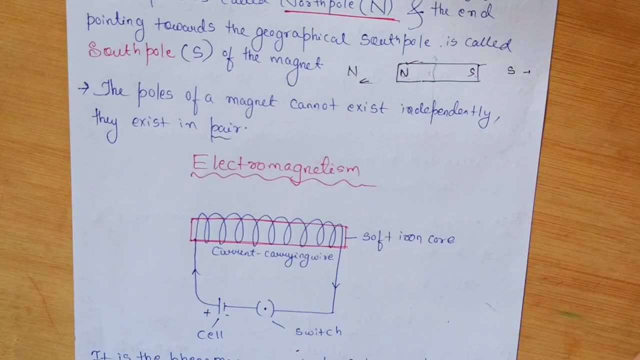 then it will be only north and south. No, Now, this part which will come will come south there. So this happens. The poles of a magnet, they always remain in pair. They never exist alone. It is a very simple thing, children. 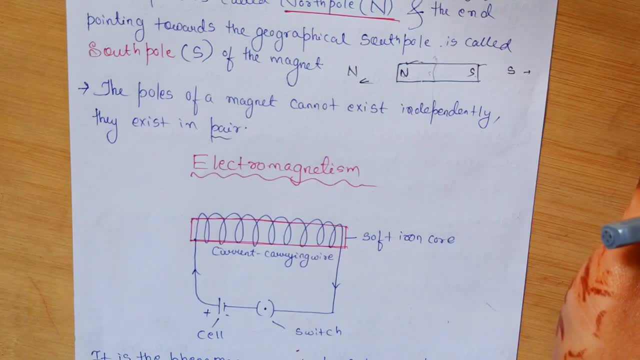 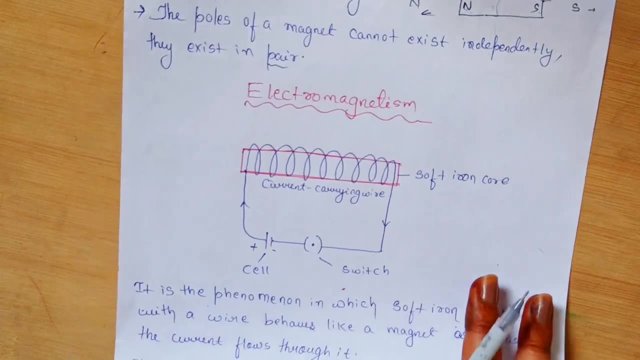 Okay, Now, after this, I gave a topic a test for a magnet, but that is basically related to experiments, So I am directly jumping into electromagnetism. Okay So, electromagnetism. Next topic is electromagnetism. Just wait. 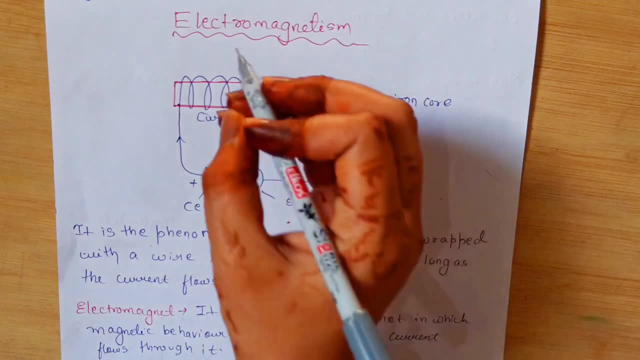 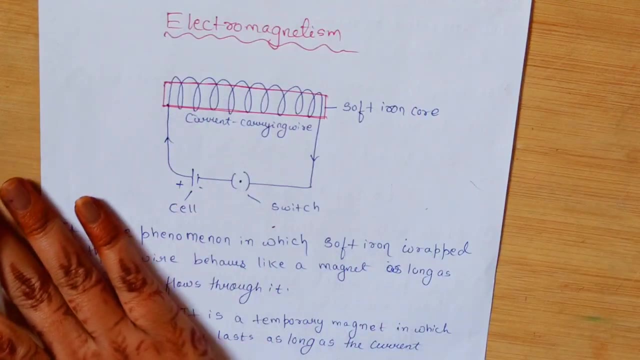 Okay, Electromagnetism. Electromagnetism means what Electromagnetism means, or you must have heard a word related to this: electromagnet, Okay, electromagnet, Okay. let me tell you the meaning of this here. 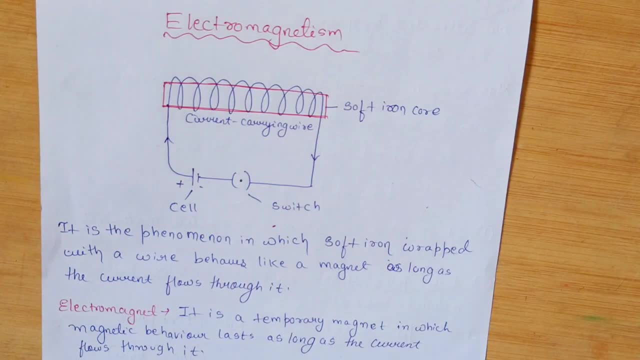 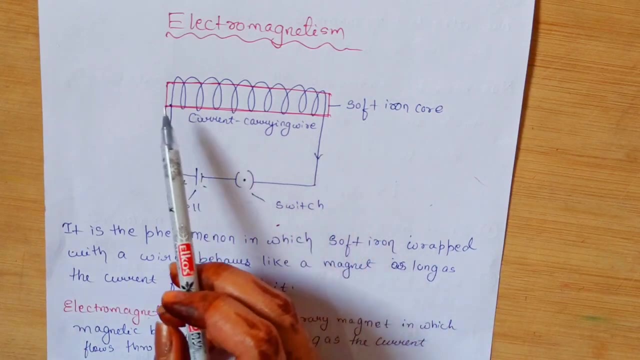 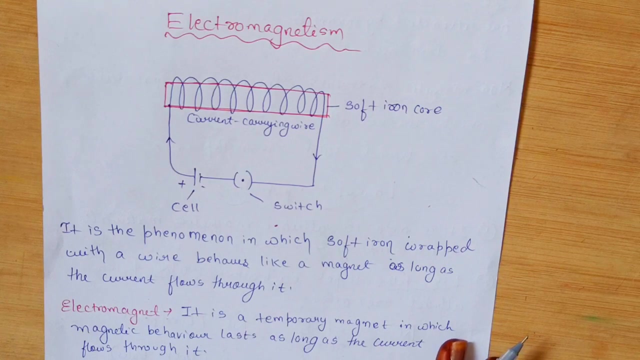 This word electro. I hope you can see it clearly, Just wait, Okay. So electromagnet. So here electro is related to electricity, Okay, And magnetism, or magnetism, is related to magnets. Okay, what happens here? Let's take a substance. 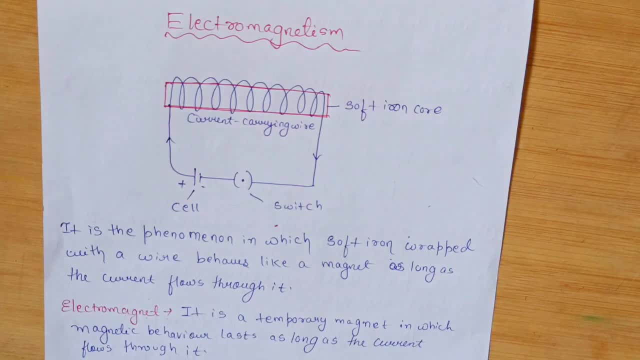 a magnetic substance. And I mean let's say we take iron. okay, Let's take iron, And by passing current all around the iron it is converted into a magnet. I mean a substance is forced to behave like a magnet. 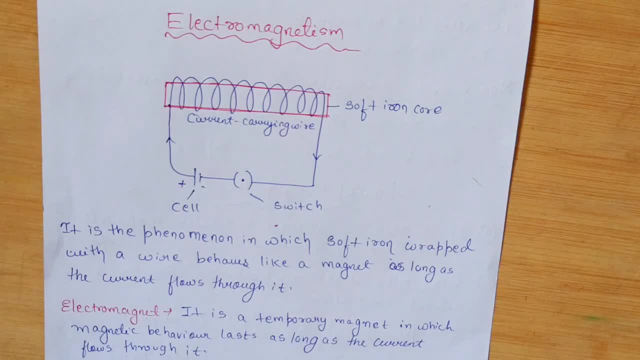 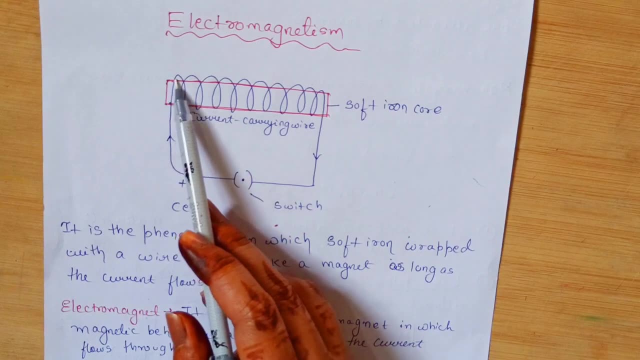 with the help of current. So we call that property electromagnetism. Let's read it. Let's read it properly. Look, Okay, look at the diagram here, children, You can see this red part. This is a soft iron core. 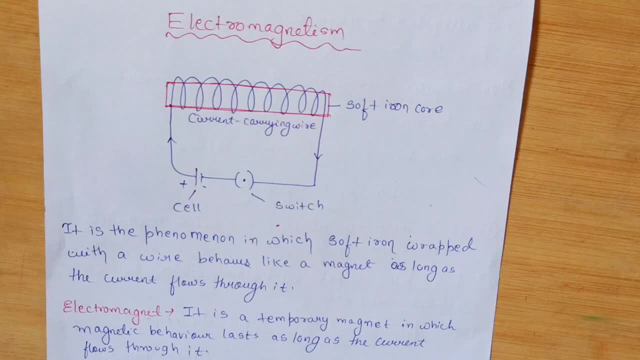 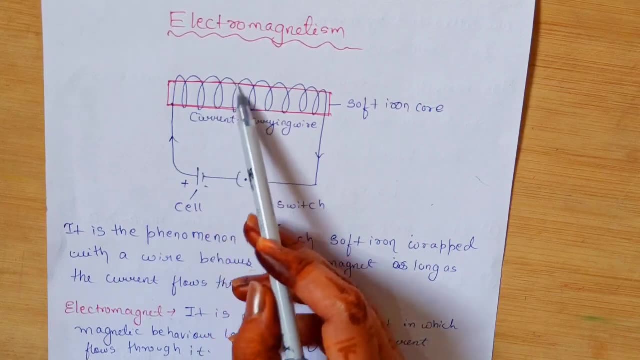 Like you have a nail, You can take that, okay. So it is a soft iron core. Okay, now what we have done is you can see this winding around it. This is a coil, This is a wire. The more you wind, the better. 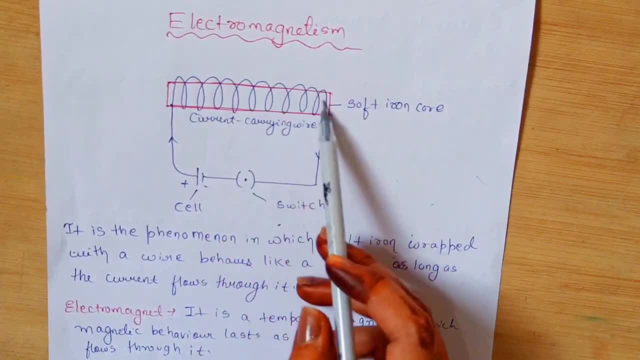 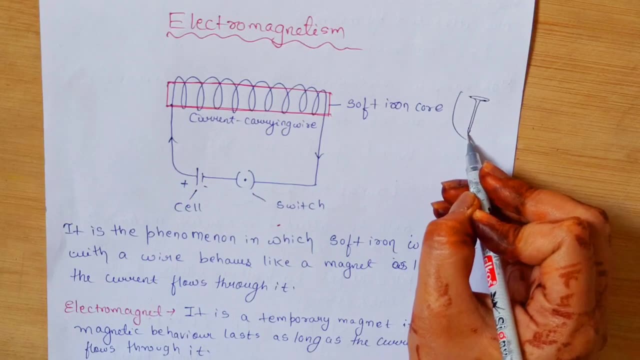 So this is a current carrying wire. This means that the wire is wrapped around that soft iron core, So in soft iron core we can take this iron. normally We can take this, okay, Actually a student experimented on this, So he took this. 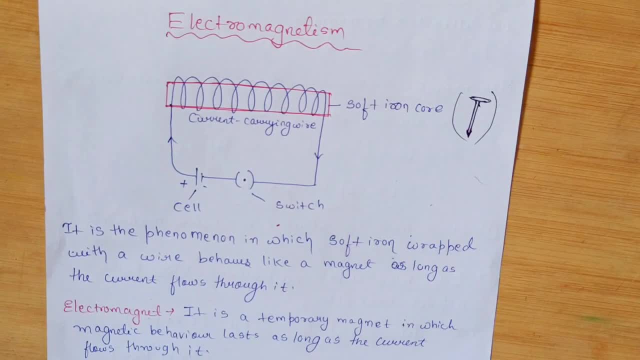 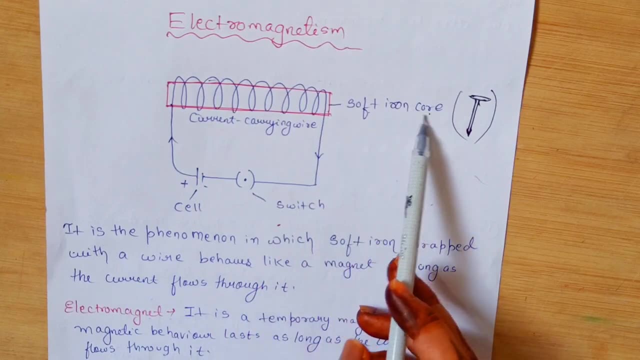 So I will make a keel here. We normally take this in soft iron core. Okay, this is a nail. okay, Okay, iron nail. So what we have to do here is, first of all, we have to take soft iron core. 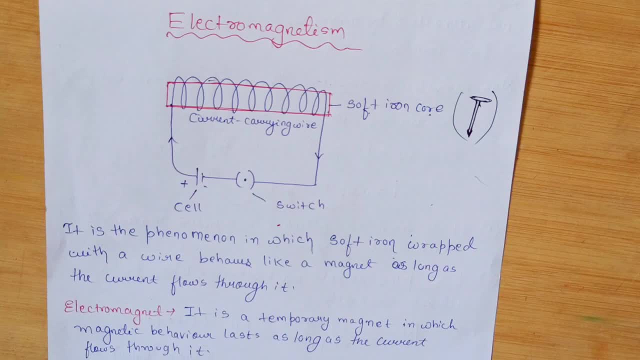 Then around it we have to wind some what You can take, a wire which will pass the current. Then there is a cell and switch. You can take a small cell, if you have a cell, Okay, And here the switch is switched on, or whatever we have to do. 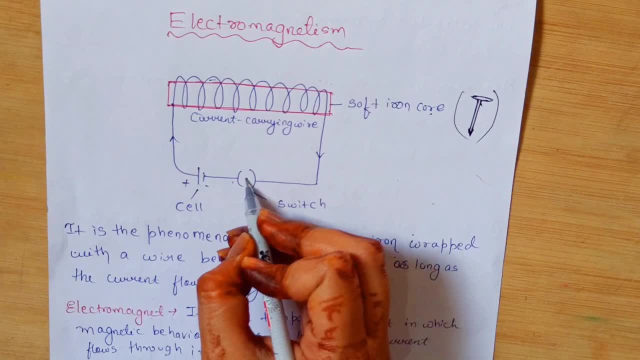 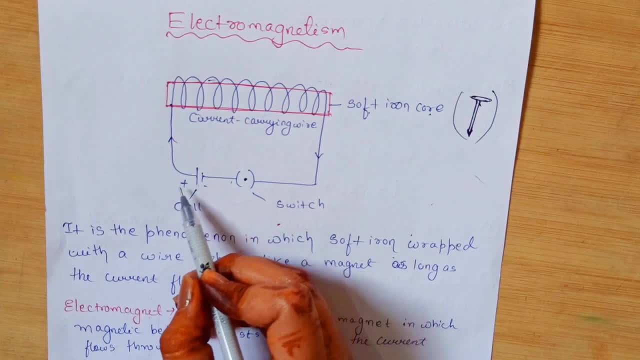 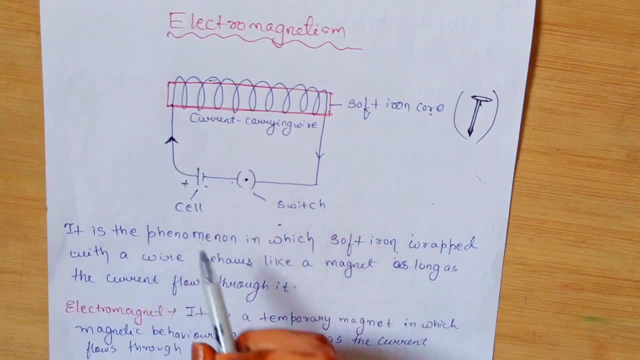 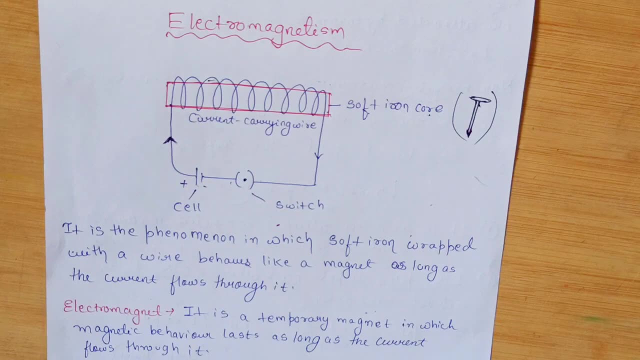 Remember this: Where the plus is seen give the direction of the current exactly. So the current is going like this and then the return is coming from here. Okay, In electromagnetism what happens is we take a soft iron, We put wires around it and make it pass the current. 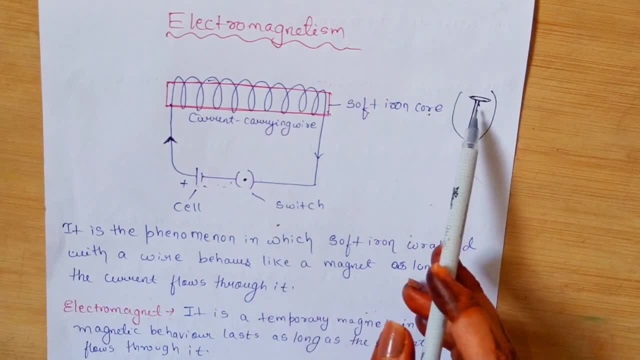 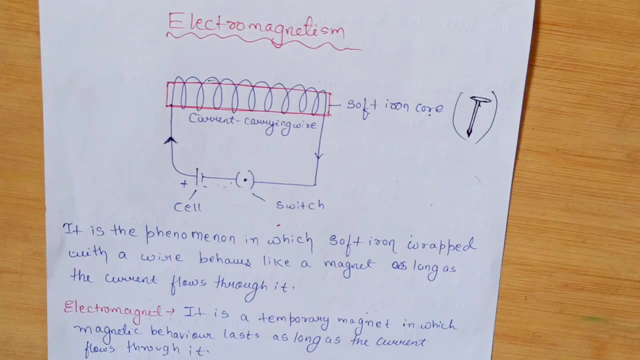 So until we make the current pass here, kids, this soft iron, This soft iron that you are seeing here, It will behave like a magnet Till the time the current will pass through it. It will behave like a magnet, But Till the time the current will pass. 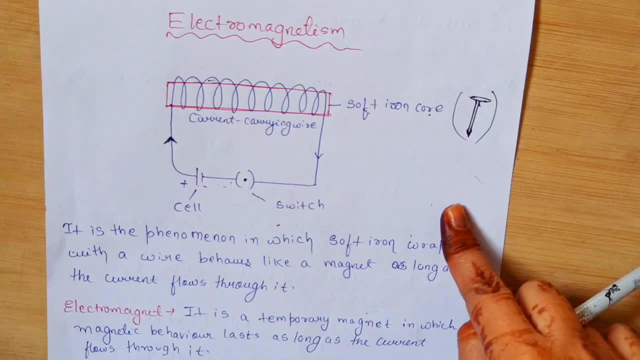 But as soon as you switch off the current, Stop the flow, It will again behave like a normal Soft iron And will not behave like a magnet. Then turn on, Then it will behave like a magnet. Then turn off, Then it will not behave. So what we have done here 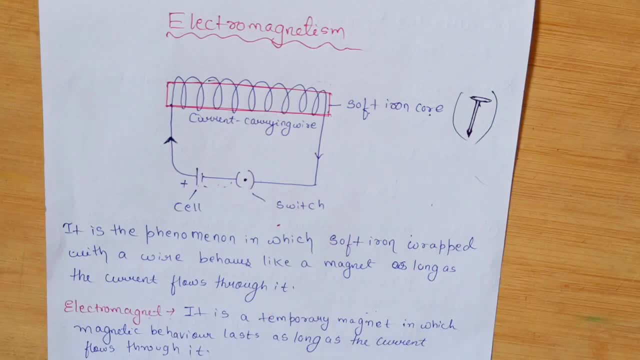 We have made a substance a magnet with the help of electricity, But till when that substance will behave like a magnet? Till the time the current is flowing. As soon as we stop the flow of the current Or disconnect the source, Then the current will stop flowing, And because of this 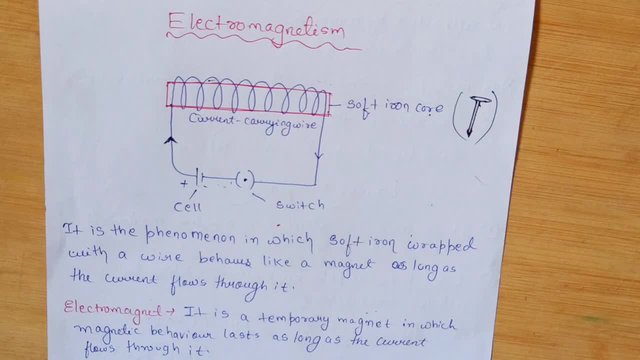 This substance will again demagnetize Means, the first one which was behaving like a magnet. Now it will not behave like a magnet. So this type of magnet Which is made, We call it electromagnet, If any magnet We are making it like this, So what we call it. 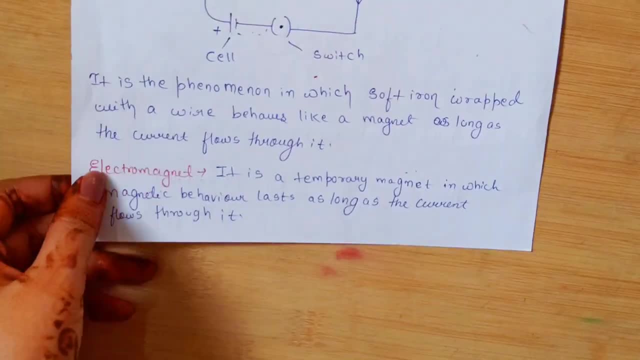 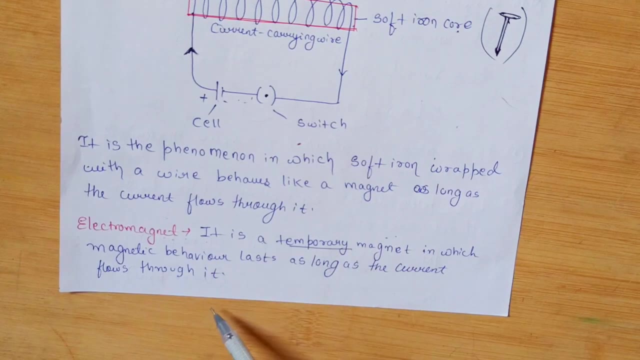 Electromagnet- Okay, Electromagnet. So let's see the definition of electromagnet: It is a temporary magnet. Electromagnet is a temporary magnet. It remains for a short time Magnetic behavior, Because Till the time you are allowing current to flow, It will behave like a magnet. 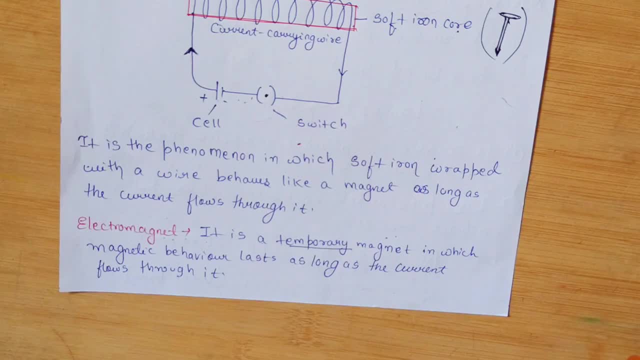 But as soon as we stop the flow of current, It will get demagnetized, Or you can say It will stop behaving like a current. Okay, So this type of temporary magnet In which Magnetic behavior Last As long as the current flows through it? Same thing, kids, Same same, same thing. 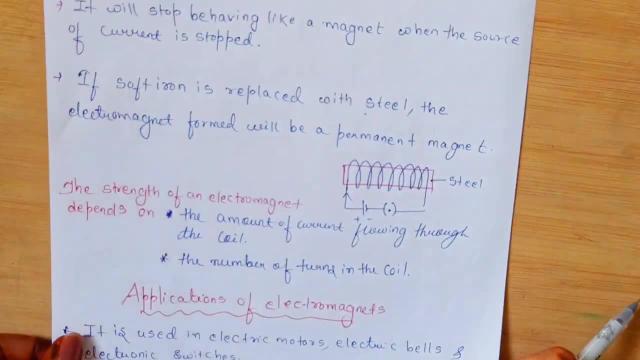 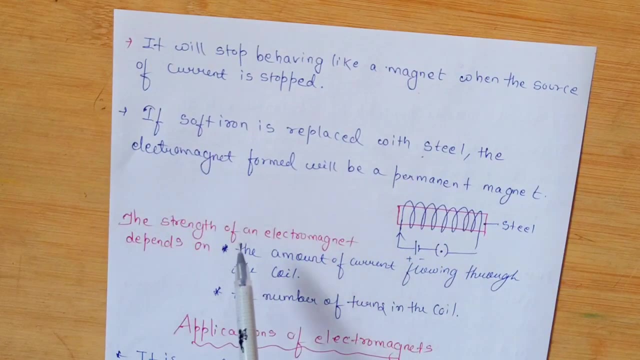 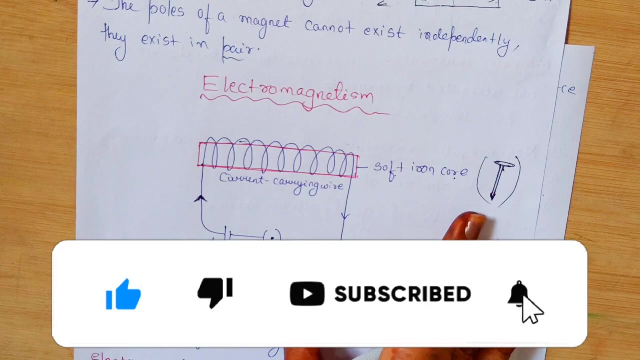 Okay, So electromagnet will stop behaving like a magnet When the source of the current is stopped. We have already told you. Now, By chance, You have another option. Suppose you are working with iron nail. Now I will tell you: Remove this soft iron core iron nail And keep a steel here. 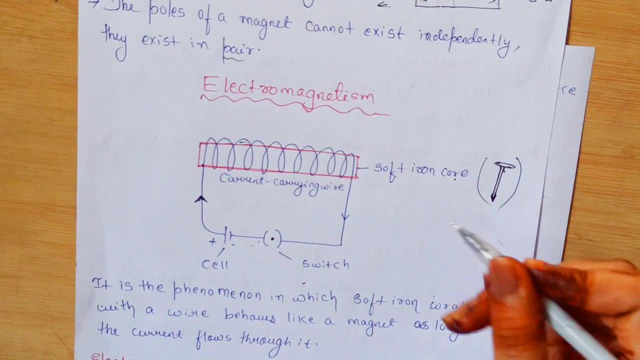 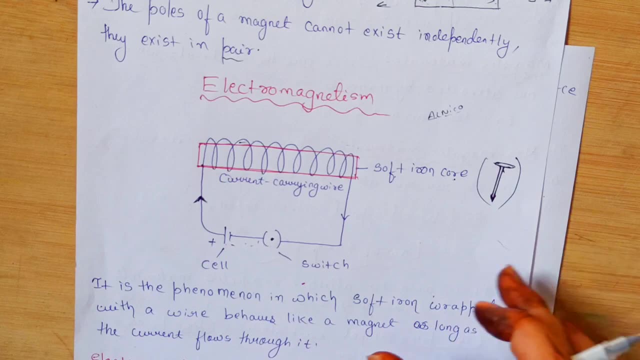 What to keep. Keep a steel, Keep a steel. We can use an alloy instead of steel. It is called Elnico. It has aluminium, nickel and cobalt. It is made up of these three things. Okay, If you don't have it in your book, Then leave it. 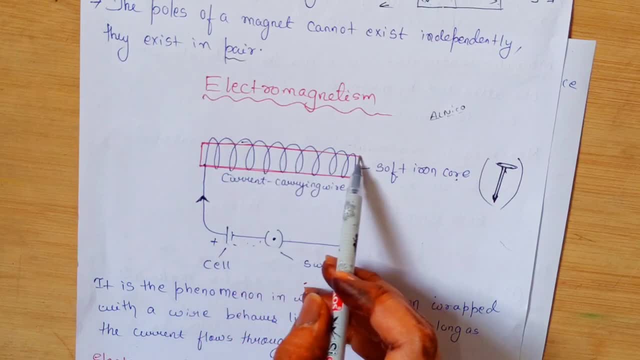 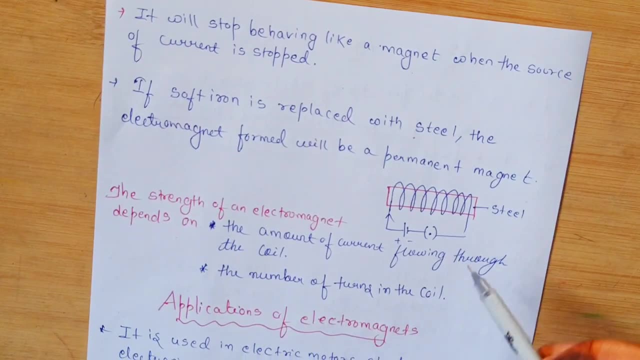 We have to keep in mind What is in the second case, If we keep this in place of soft iron core? What will we keep? We will keep steel. So what will happen When the current passes here? Because of that, Steel will behave like a magnet. It will become a magnet. 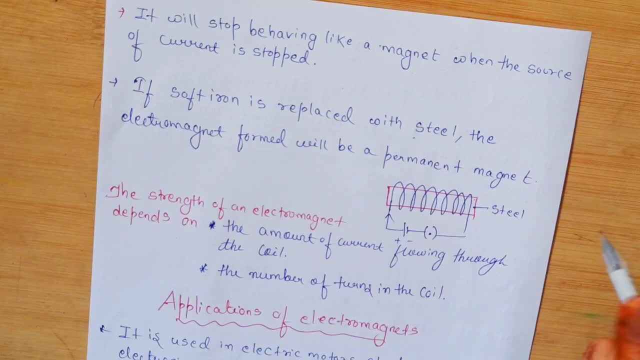 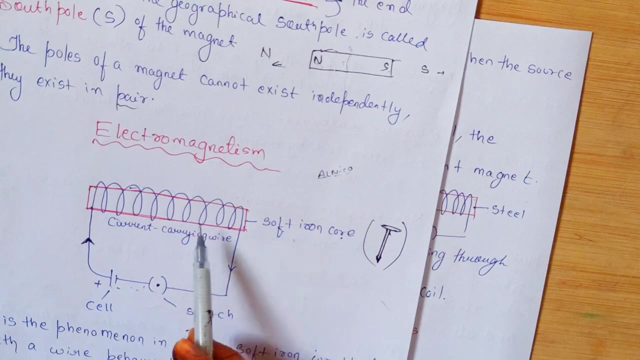 If we switch off too, It will not lose its magnetic power Or magnetic behavior It will not lose. Okay, So if we replace soft iron with steel, The electromagnet that will be made here We will call it permanent magnet. But when we were taking soft iron core, When we were taking this soft iron core, 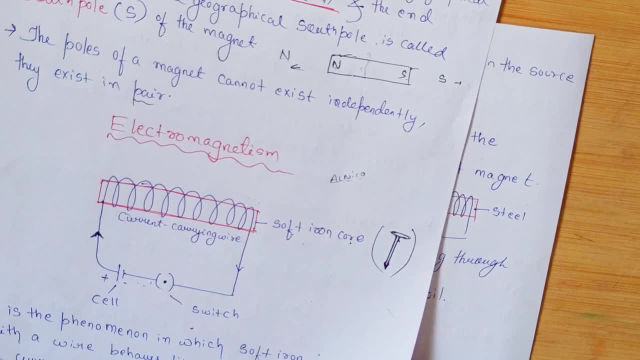 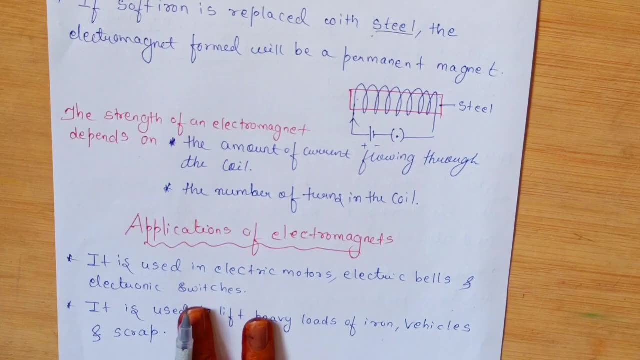 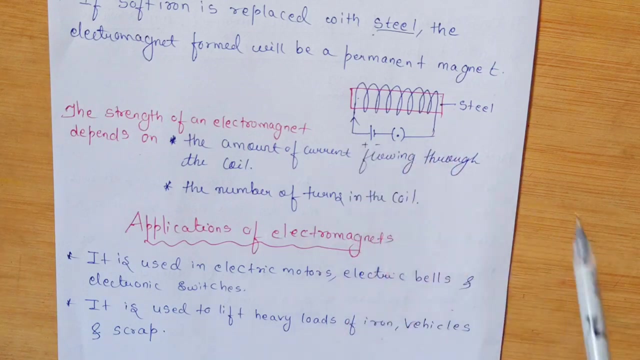 Here it was behaving like a temporary magnet, But as soon as we replace it with steel It will behave like a permanent magnet. What kind of magnet? Permanent magnet? Now, the strength of an electromagnet depends upon, Now, the strength of an electromagnet. How powerful is its strength? 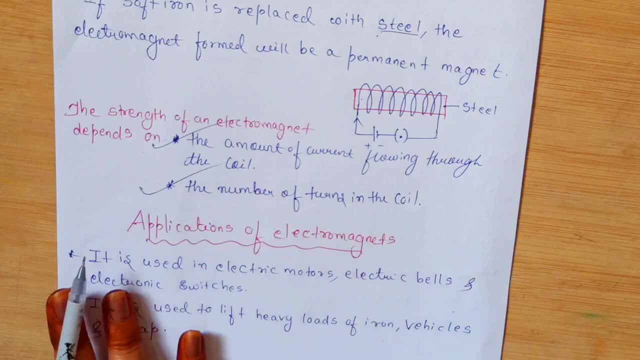 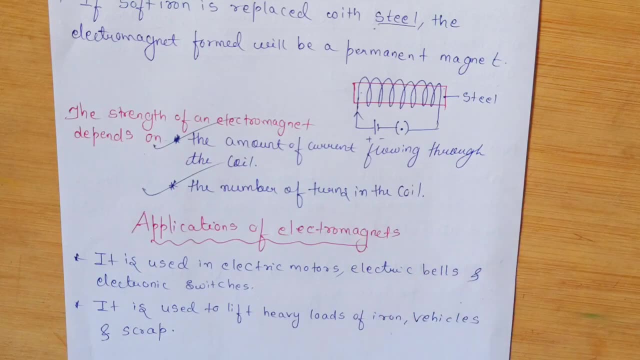 In which it depends. This is very important. It comes in very important exam. Okay So the strength of an electromagnet: It depends upon two things. First, amount of current flowing through it. How much current are you passing? If you pass more current, It will have more magnetism. 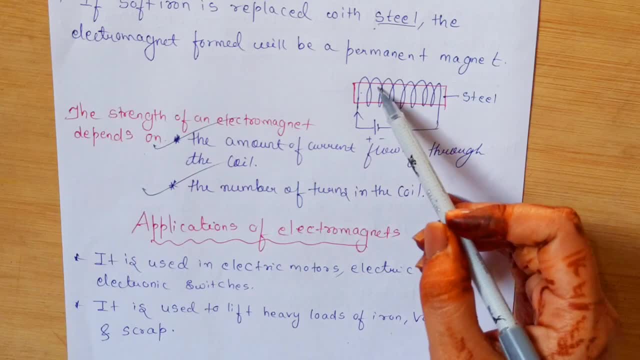 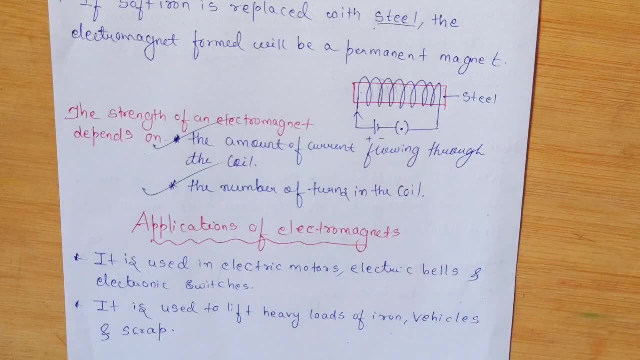 Right, It will become strong. And the second factor is number of turns. The number of turns in this Means the more you wrap the wire in this, The stronger magnet will be, The more strong magnet you will get. So there is nothing much in electromagnetism and electromagnetism. 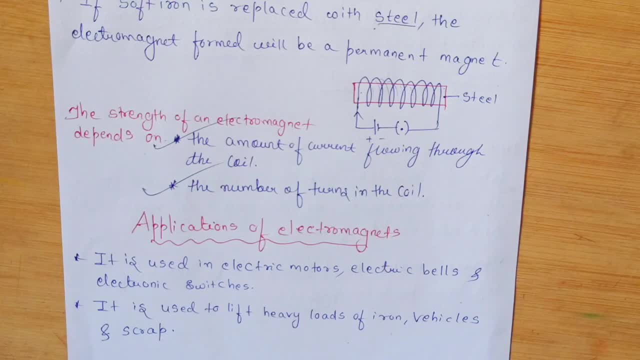 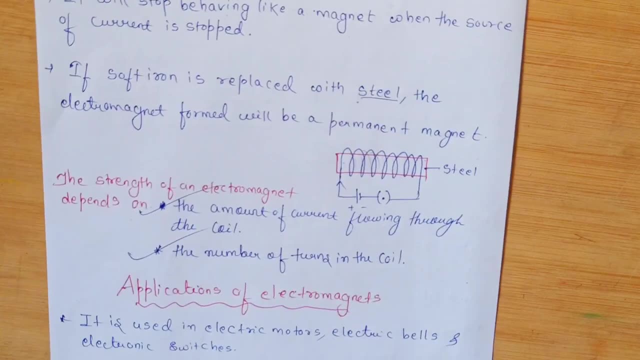 It is a very simple thing, So you have to remember that. Okay, I am also looking in the book. It is written as: special alloy in the book Means if we replace the soft iron with steel Or an alloy whose name I told you, Elnico. So I will write it here once. 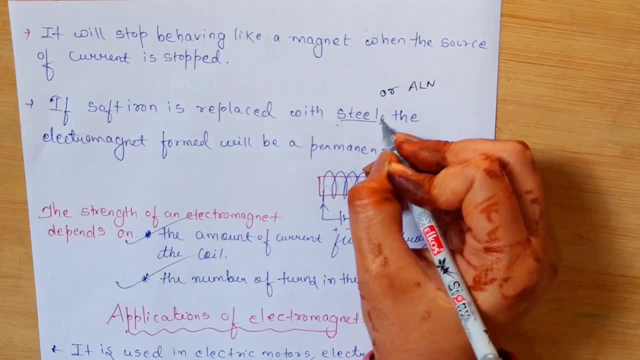 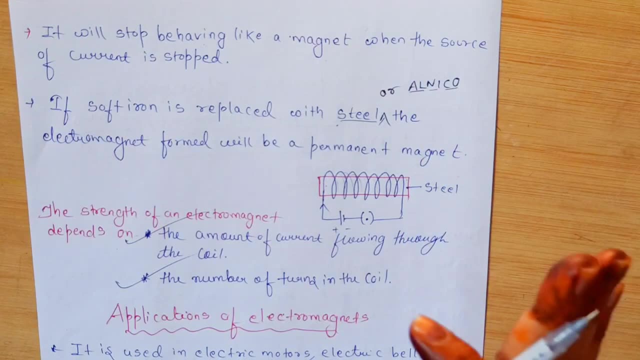 And Elnico. Okay, and Elnico. So remember Elnico. Al means aluminium, Ni means nickel, Co means cobalt. So we have to use these three And make an alloy. We can also keep it in place of a soft iron. So what will we get? 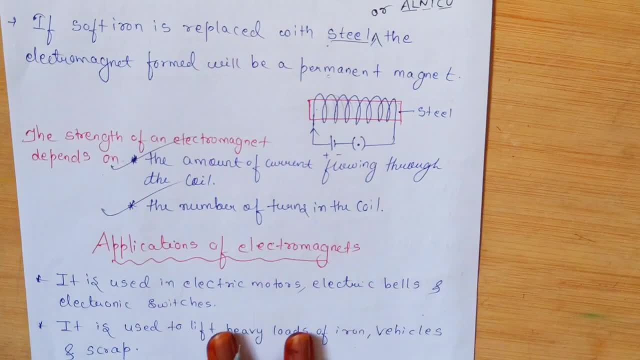 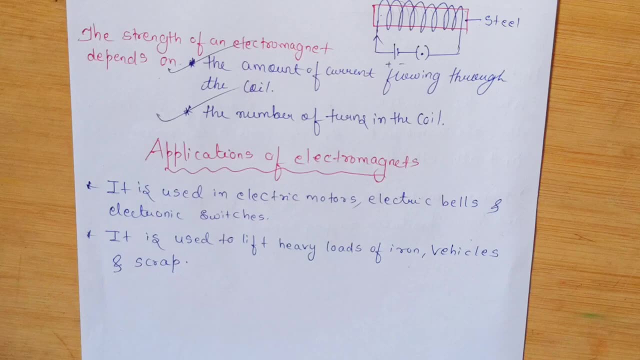 Electromagnet. Definitely we will get electromagnet, We will get permanent magnet. Okay, Now let us look at some applications. Not much. If you have given more, Then you have to read these. I am telling you only two points. Application of electromagnet: Electromagnet has a lot of applications. 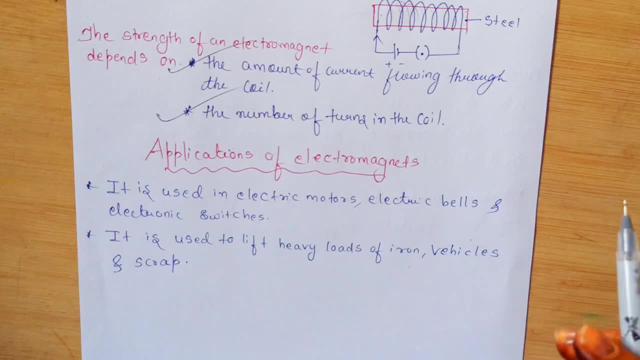 A lot Means. It is basically used in the electric bell- Which is our door bell- That is what we call it- in which this thing comes electromagnet. its phenomenon is used in switch in electric motor. it is used to lift heavy loads of iron vehicles and scrap. 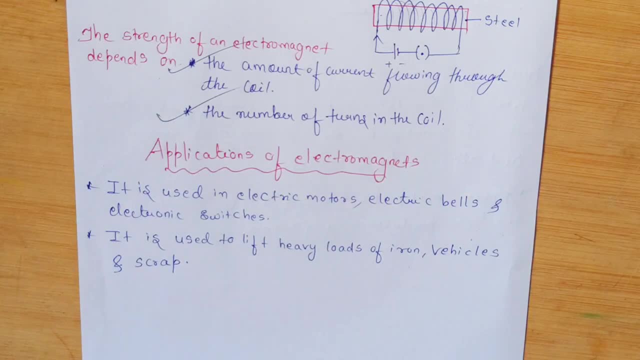 means, suppose, if I say that there is a very heavy load of iron, we have to lift it, lift it, then electromagnet is used there, like there is a lot of garbage, and if there are a lot of iron particles in the garbage, then the crane also uses this phenomenon. 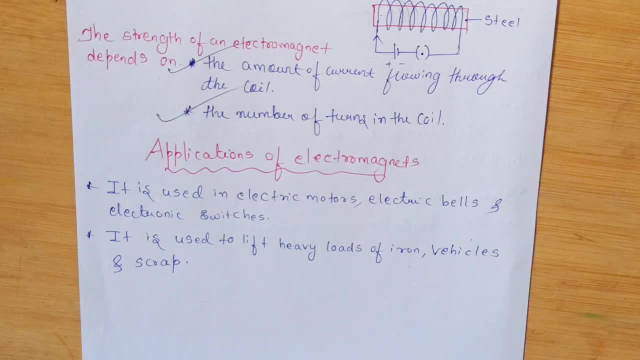 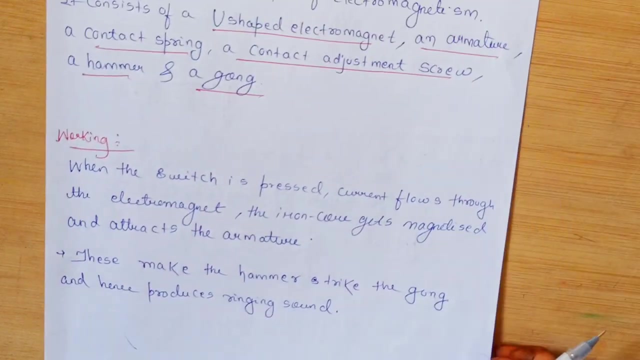 it separates all the iron or magnetic particles, like there are a lot of them in mining industries also. it is used to separate iron ores. to separate iron ores. it is used in mining industry. you can read about this in higher classes. there is more or less then electric bell. 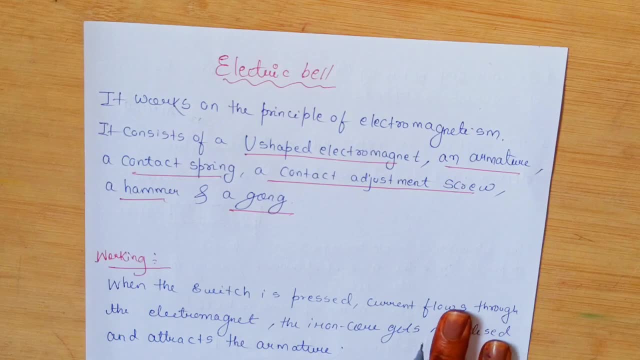 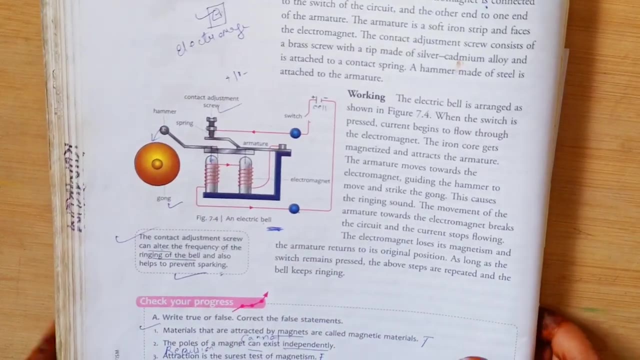 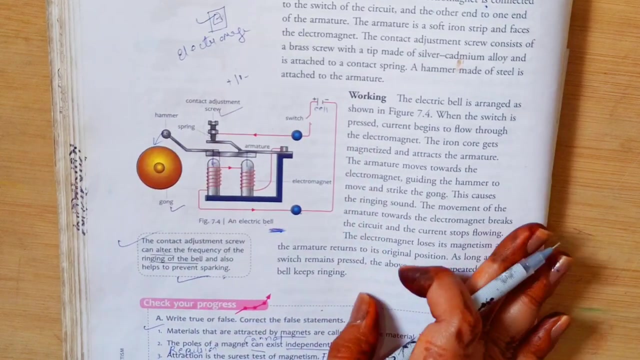 electric bell. see what is electric bell. I have not made a diagram of electric bell. I will show you from books only. ok, this one. this is electric bell. ok, see what is in electric bell. I have just told you that the electric bell works according to the principle of electromagnetism. 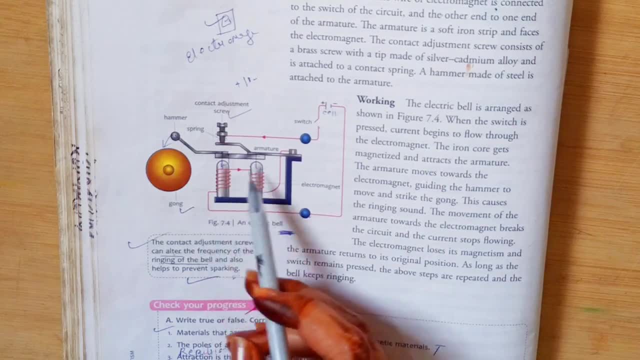 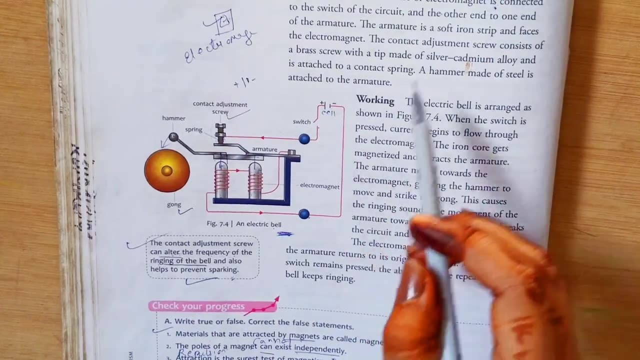 means same. we will pass the current, so the things we have taken here- it will behave like a magnet. as soon as we switch off the current, that thing will not behave like a magnet. so it works on the principle of electromagnetism. so here you can see. 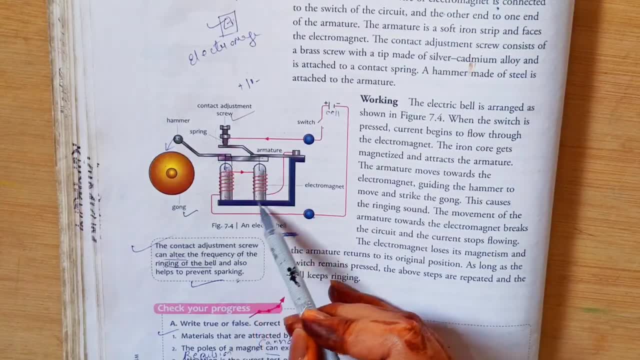 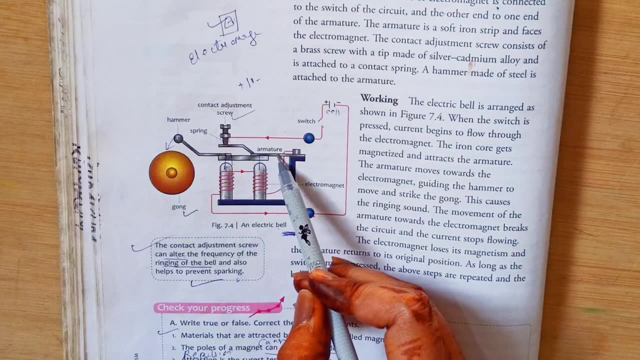 there is a U shaped electromagnet. you can call it U shaped electromagnet. proper U is not visible, but you will consider it as U. ok, then after that, here is armature. ok, armature is made up of one type of substance. then here you can see a spring. 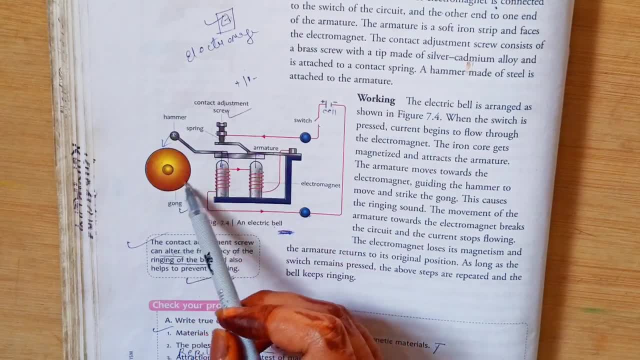 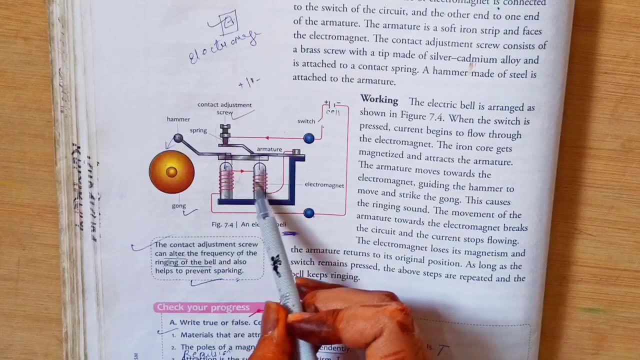 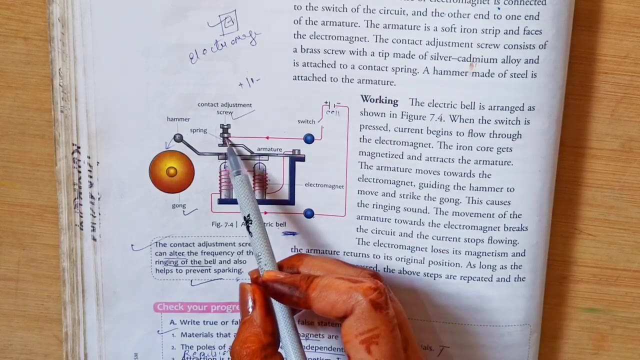 this is a contact adjustment screw. then here is a big gong, it is attached to the hammer. you cannot say attached hammer is attached to this. then here wire is wrapped around this U shaped electromagnet. then one end of the wire is connected to the cell and the other end is connected to the switch. 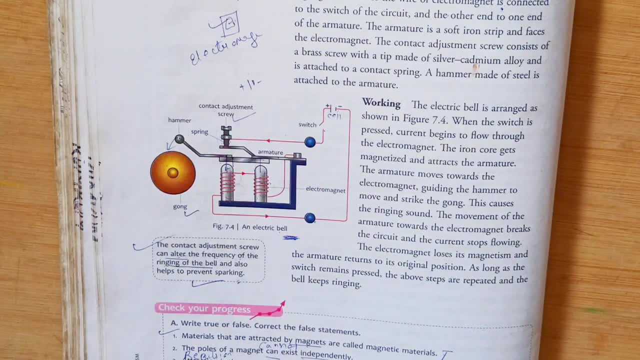 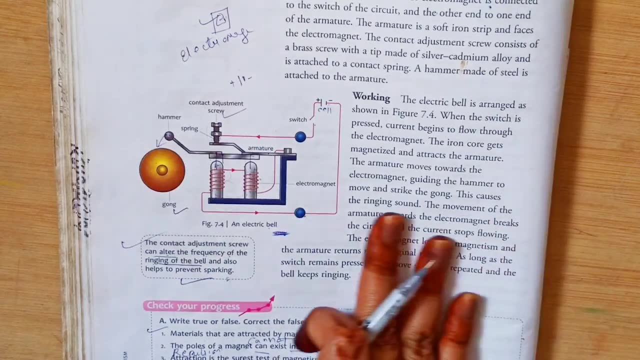 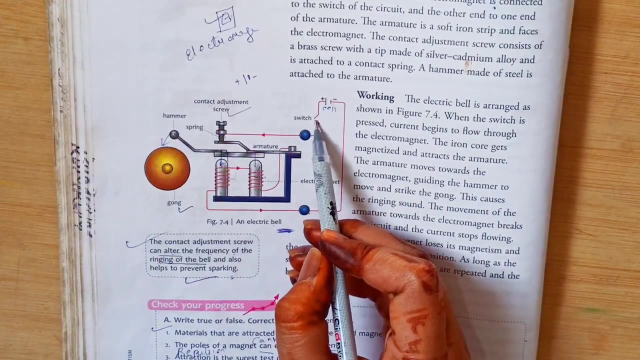 from the contact adjustment screw, like this type of arrangement is given here. ok, now directly, we will see its working. so there is nothing in working. see, it is very simple. now suppose someone comes to your house and he switches on. when the switch is on, then it will be attached to this. 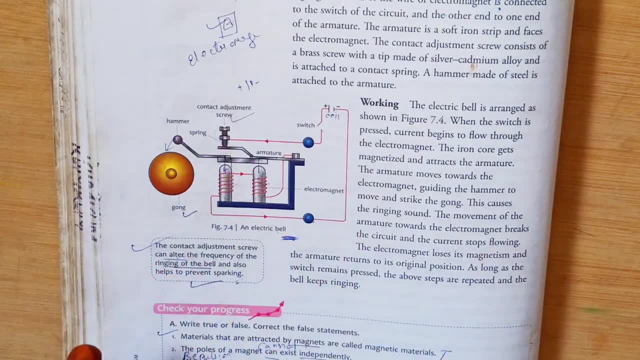 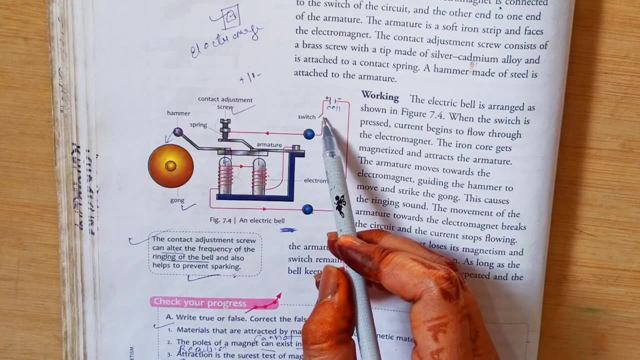 means when it will be attached, then the circuit will be completed, then the current will flow. ok, so when anyone presses the bell here, if you press the bell, then when the circuit is completed, then the current will flow. obviously it will flow. and see, here is plus and minus. 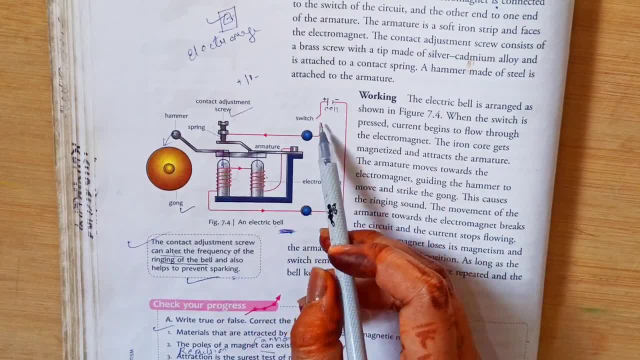 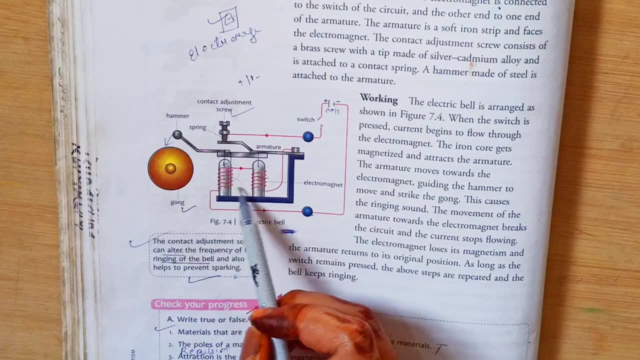 so make the direction of the current from the plus side. ok, now the current will flow here. see, the wire is wrapped around it right. so due to the flow of current, this part- it will behave like an electromagnet. how it will behave like an electromagnet, ok. 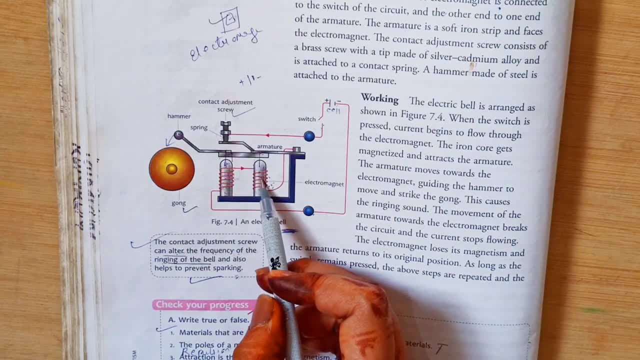 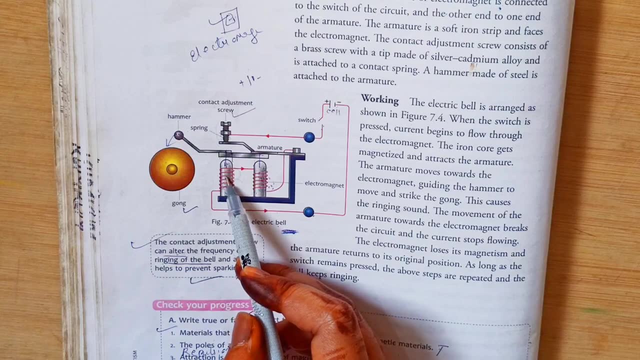 it will behave like a magnet, so it will be magnetized. it will be magnetized, so it will be magnetized. see it. draw down now you can see. it will pull the armature towards this. armature will pull towards itself when it comes towards it. so this hammer. 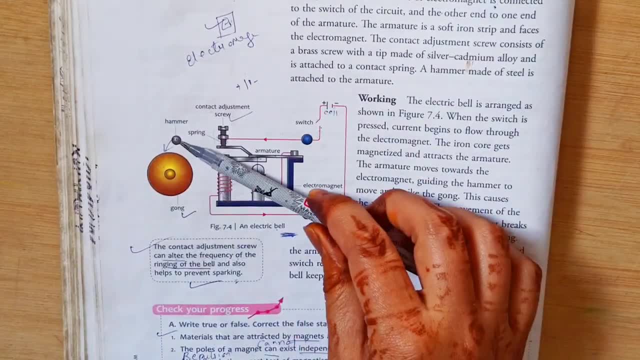 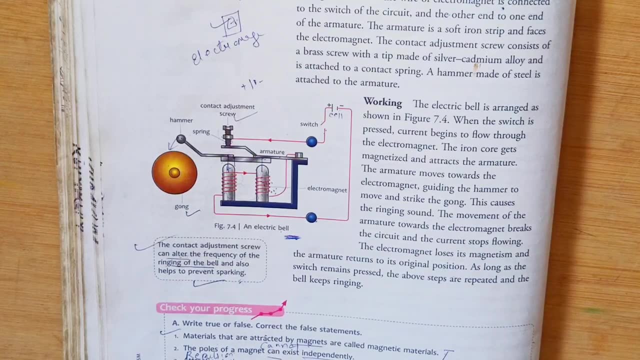 see if the armature will bend down towards the electromagnet so definitely, the hammer will also come down and will strike at the gong and there we will hear the bell. and as soon as we switch off and release the light, then the sound stops till you keep the switch pressed. 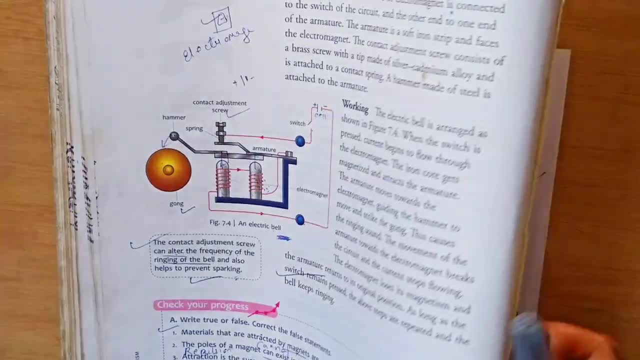 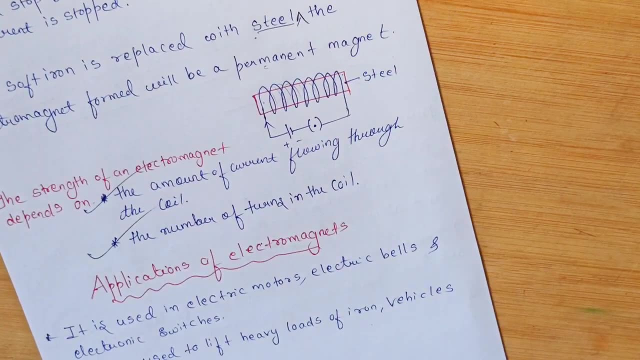 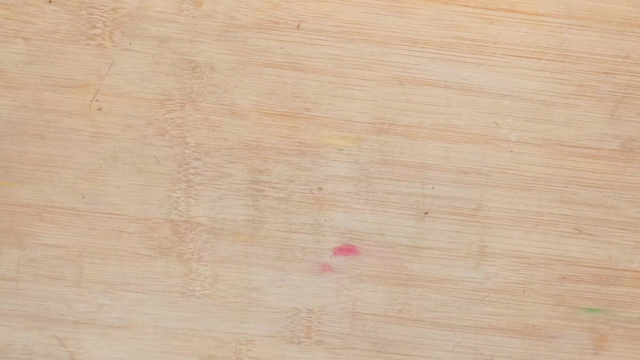 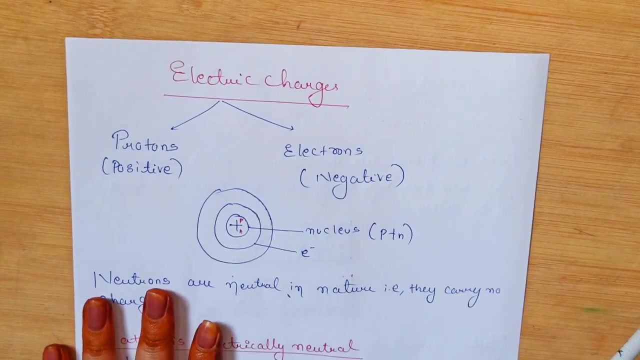 the same step will be repeated and the bell will keep going. ok, it is very simple. so i am explaining here in a very simple way. i even wrote it very short: book se bata jiye aap logon to. Okay, Then uske baad hai electric charges. Okay, Ab bacho. 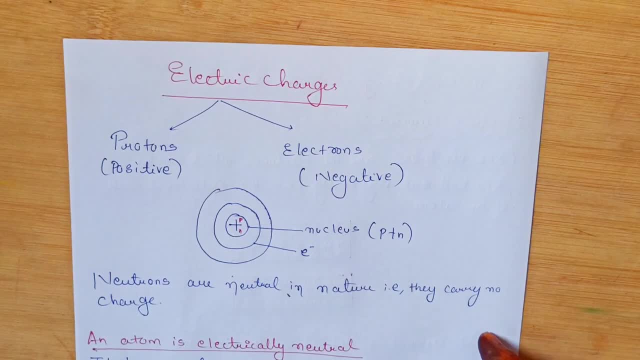 dekho electric charges. Matlab, ye electric ka charge ka baat kar la. Ye already aap noko thoda baat pata hoga. Chemistry me toh padta hai, hum logon iske baare me Acha Electric. 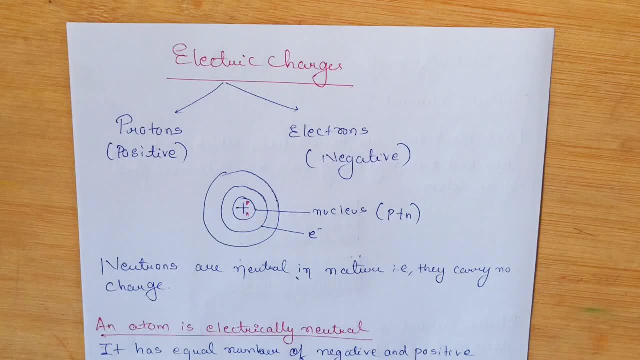 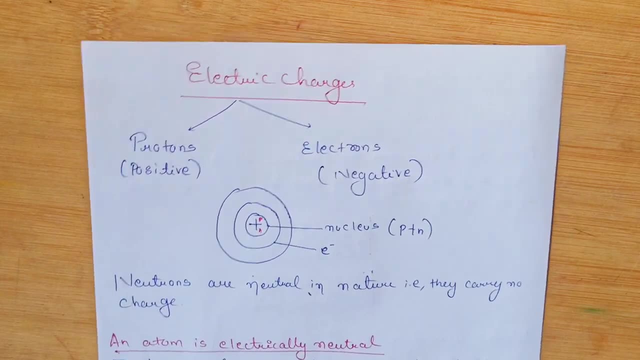 charges me: kya hai bachho? dekho Basically bachho. duniya me is, universe me. jitne bhi objects hai, Hum sab pade hai, ki they are made up of small atoms. They are matter. Sab toh matter nahi hai, but jo bhi matter hai, wo logon atoms se bane, bhe Hena Itam simple. 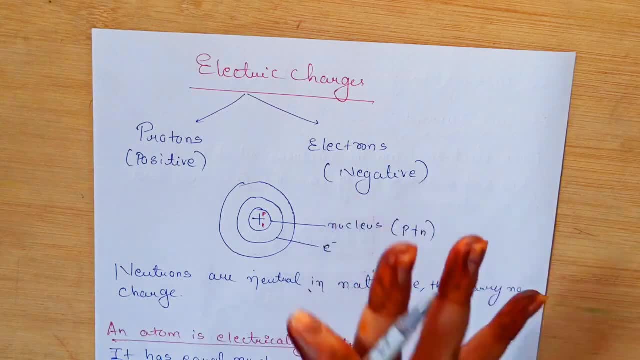 tha jeet hai Class 6, se aap logon ko padhate aayi hum. So all objects in this world are made up of atoms. Small, small atoms. Acha Atom aisa dekhta hai. Ye, toh aap logon ko pata. 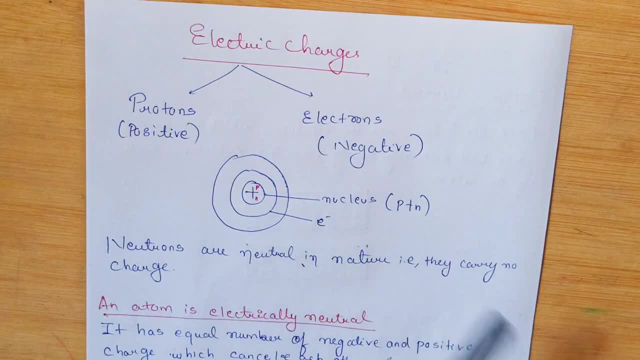 hoga. atom kesa dekhta hai. Thike Humare koi bhi object bhi la Aap logon ki paan hi lilo Isme kitne saare atom hongi hum gin bhi ni. 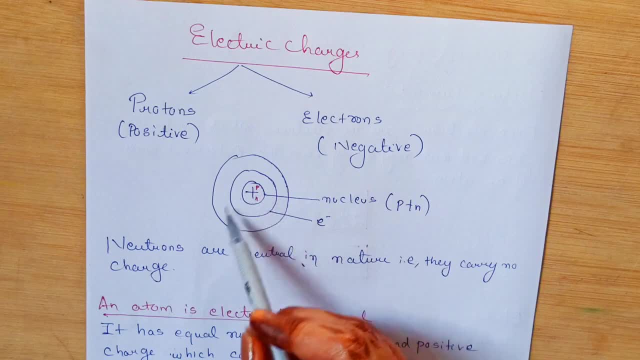 Itse atoms hote hai present Har object me Acha Aap atom ko ek baar dekhlo. Atom ka ye jo beech wala part hai, jaha, par mai plus banayi ho, Ye whole part, hum nucleus bolte. 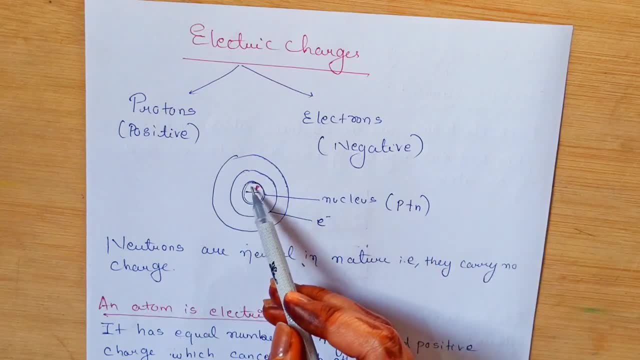 hai Kya bolte hai: Nucleus, Iska naam hai. Thike Uske bahar, aap logon, dekho, ye toh nucleus ho gaya. Uske bahar ye aap logon koi jo gol, gol structures dikh rahe hai. These are called. 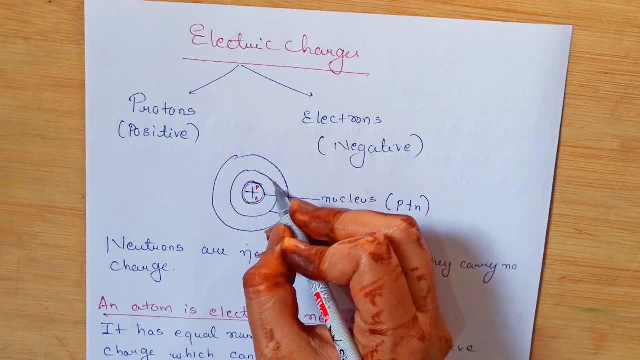 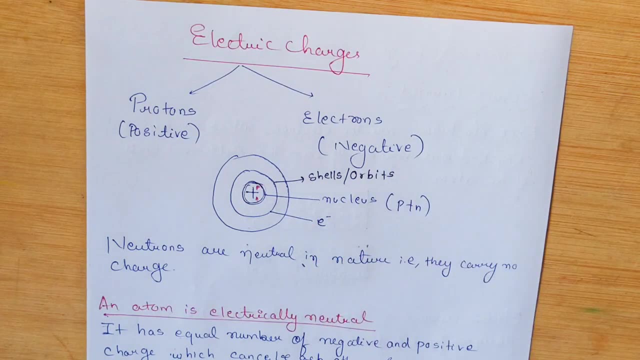 shells, Isko shells. mai aapar mention nahi kar rahi hu, but mai kar de rahi hu. These are called shells or orbits. Ya toh shells bolo, ya phir orbits bolo. Acha Abhi Ye jo atom. 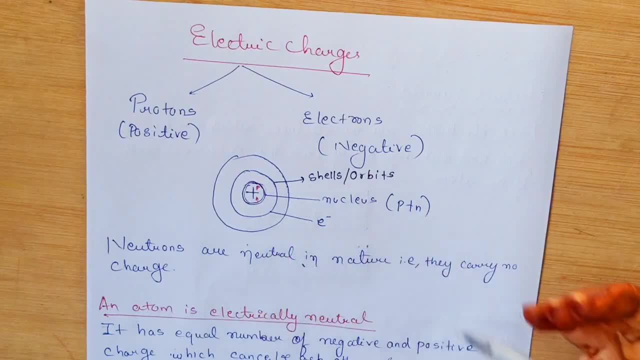 hai. yaha par na Tien particles hota hai, Tien cheez hota hai, Ek hota hai electron, Ye raha. Ek hota hai proton Aur ek hota hai neutron, Thike Electron, protons and neutrons. But yaha par. 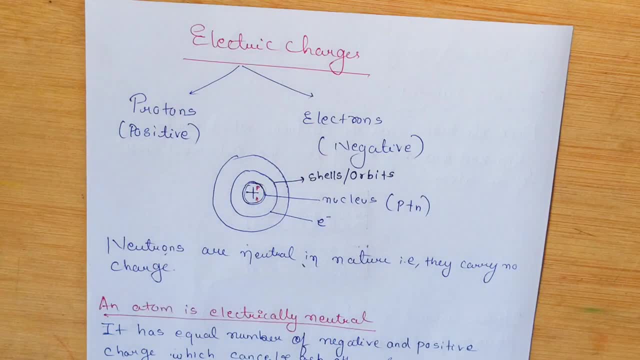 charge ka baat ho raha hai, Charge toh important hai, Toh charge neutron me nahi hota. Charge hota hai present electrons and protons me Thike Normally jo humne electrons, protons, jo word use kar rahe hai, Ye kuch aise particles hota hai, jinme kuch charge hota hai Toh protons. 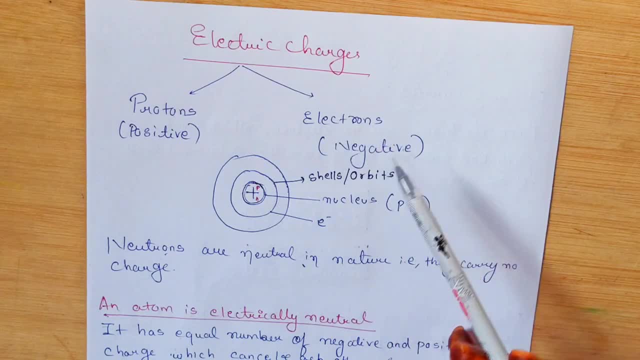 ke paas hota hai positive charge and electrons ke paas hota hai negative charge. Acha Abhi ye jo proton hai, Wo raheta hai nucleus ke andar me. Aap loko dikhta hoga mai aapar small. 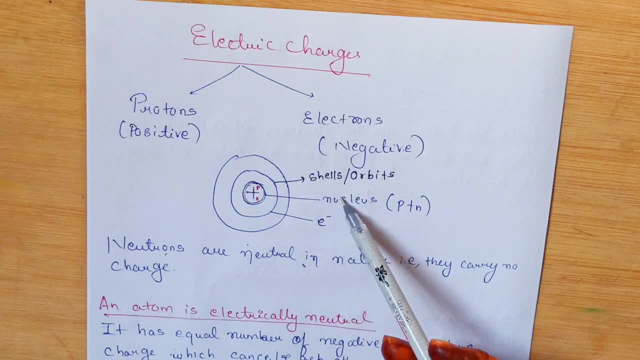 sa pili ki hoon, Toh nucleus ke andar me rahega. proton. Tike Acha Abhi ye jo neutron hai. Iska toh koi charge nahi hai Par ye bhi yahi par raheta hai, Proton ke saath bolta hai. 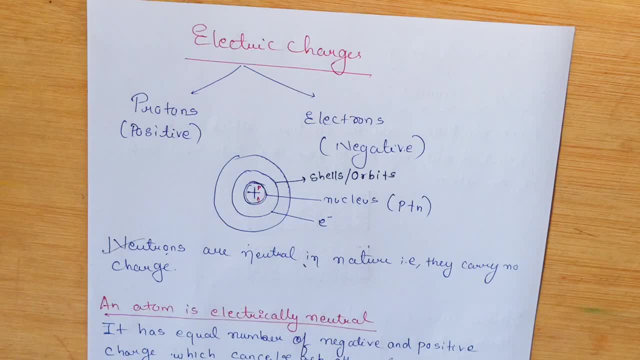 mai adjust kar lunga. Aur wo araam se proton ke saath nucleus ke andar me matlab raheta hai. Acha, Ab baat karte electrons ka, ki electrons jinme negative charge hai. bolo, kaha, rahetay hain Toh electrons ghumte, rahetay hain shells me. Ye jo shell dikha raha hai. 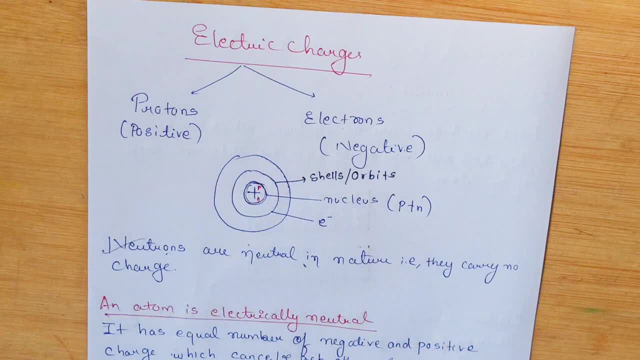 Ye orbit dikha raha hai, Yehi par ghumte rahetay hain. Yeh shell dikha raha hai, Yeh shell dikha raha hai, Yeh shell dikha raha hai. Yeh orbit dikha raha hai. Yehi par gol, gol, gol, gol electrons. 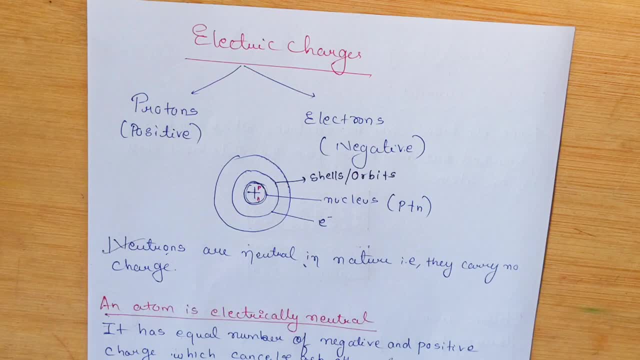 lunga, Kya karte hain. Ghumte rahetay hain Aap, kaun se orbit me kitane electrons hongi, woh sab higher classes me, Kyunki kuch, kuch bachcho ko doubt raha hai, ki hum logo ko kaise. 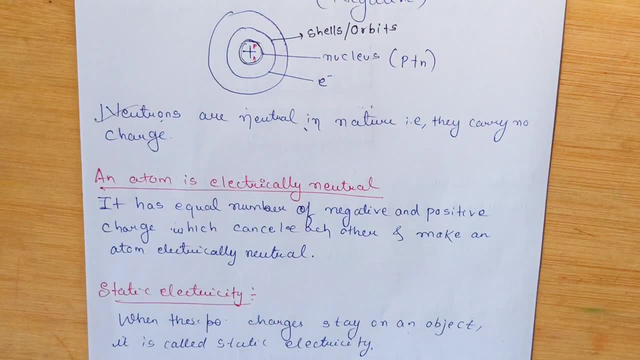 pata chalega ki electrons kaun se shell me ghum rahe hai. Kitane hai jozi Tike, Wo bat ka baat hai. Acha, Abhi Aap dekho, Aap logon ko maine bata diya ki protons and neutrons 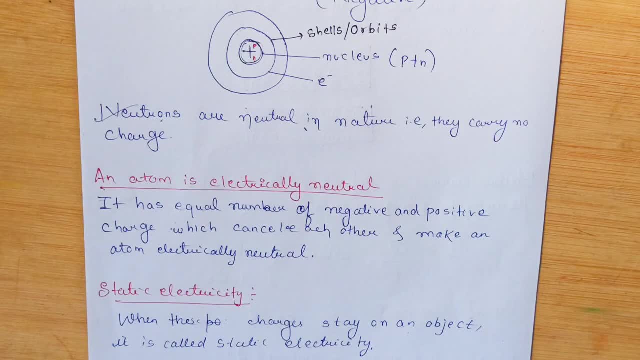 pahe jate hain. nucleus ke andar me Electrons jo hota hai, wo shells me ghumta hai Neutron. There is no charge of electron, but there is mass and weight. negative charge of electron, positive charge of proton. weight of electron, but the mass is nearly negligible. 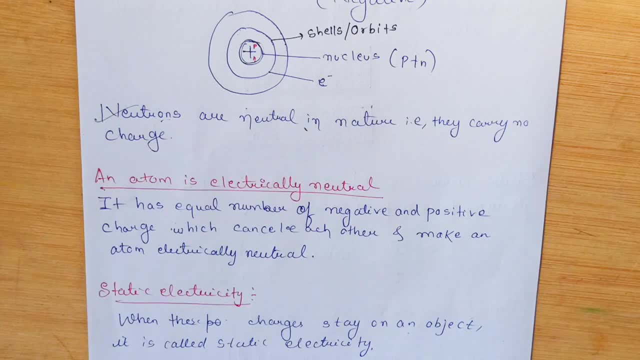 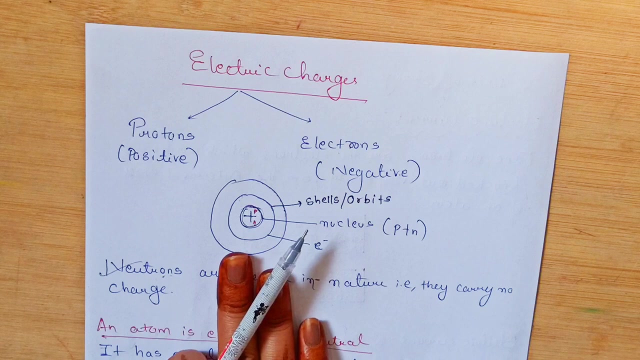 Means we can consider it as massless. Normally what happens is, if I say: under normal circumstances an atom is electrically neutral, Atom is electrically neutral means, as you can see here there is an atom. Electrically neutral means there is no overall charge in it. 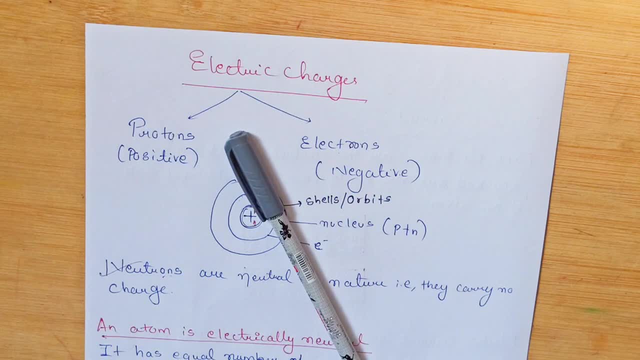 Consider this pen as an example. There will be a lot of atoms in it, So the overall charge of those atoms is zero. Suppose this pen is an atom- And what is an atom? It has overall zero charge Means it is neutral. 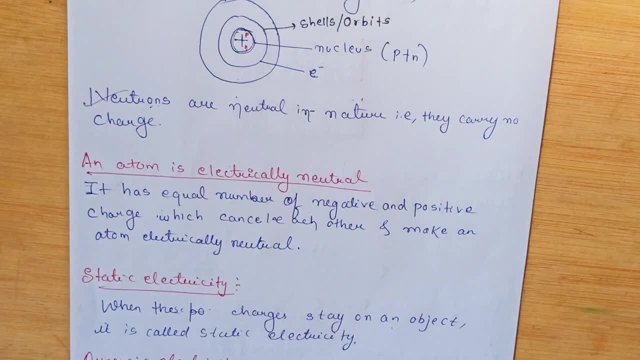 So here the same thing has been told: That an atom is neutral. Why is an atom electrically neutral? The reason for this is that in every atom what happens in normal condition? In every atom, the number of electrons and protons remains equal. 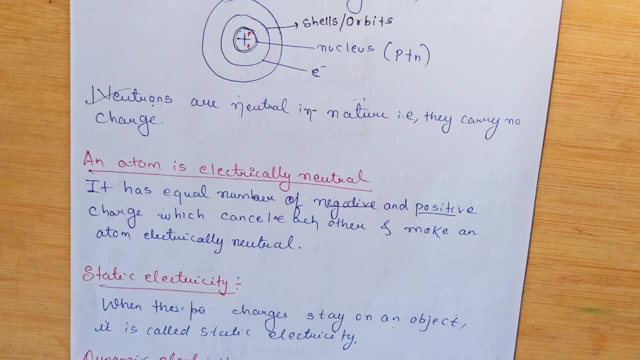 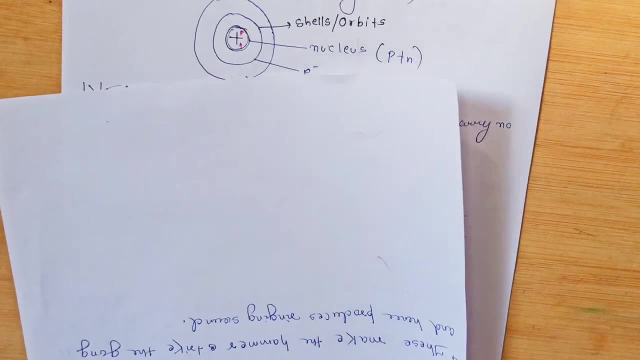 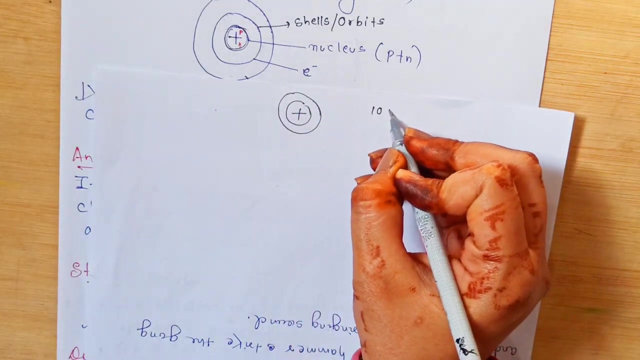 Means the number of negative particles and positive charge particles are equal. Let me tell you an example. Let me tell you here: Suppose there is an atom- I am making it normally- Suppose there are 10 electrons and 10 protons in it. 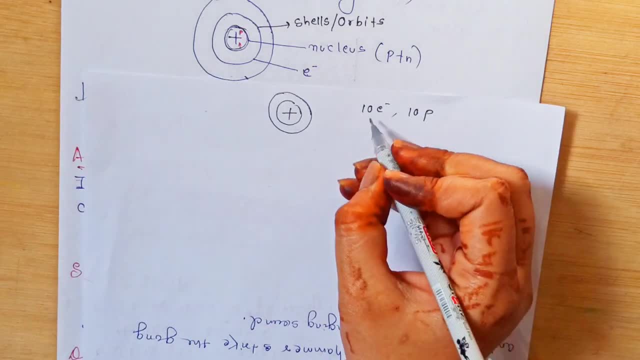 10 electrons and 10 protons. So this 10 is of minus 10 electrons: 1,, 2,, 3,, 4,, 5,, 6,, 7,, 8,, 9, 10.. 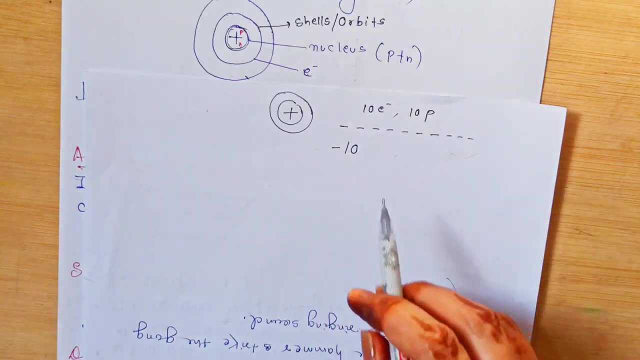 I am not making it like this. I am writing it directly like this: Minus 10.. Minus 10 means there are 10 electrons Minus charge is there, I have shown minus And there are 10 protons in it. 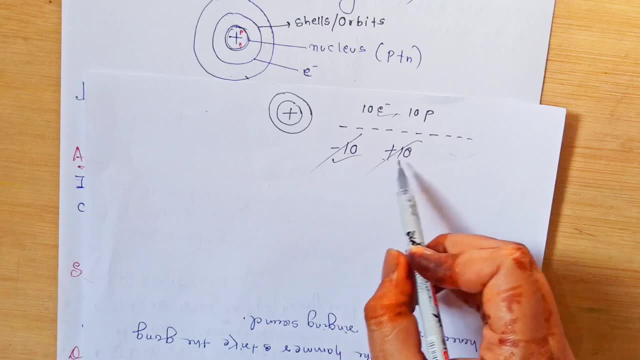 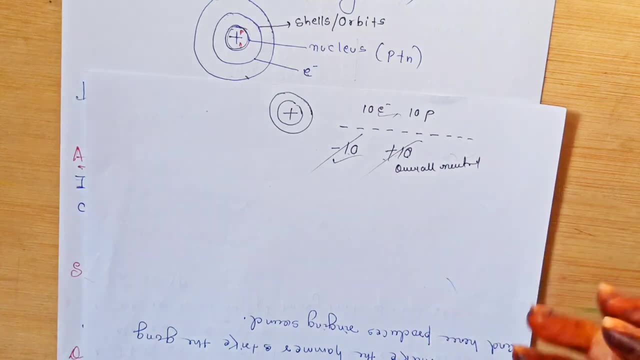 So what is the charge of protons? It is plus, See, it is plus minus, Minus 10 plus 10 is zero. So that is why we say overall no charge, Overall electrically neutral. Okay, This is an atom. 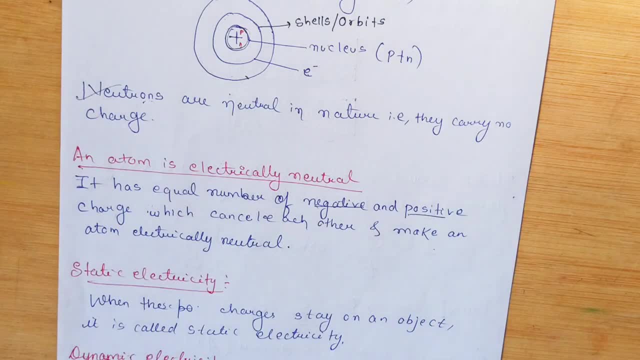 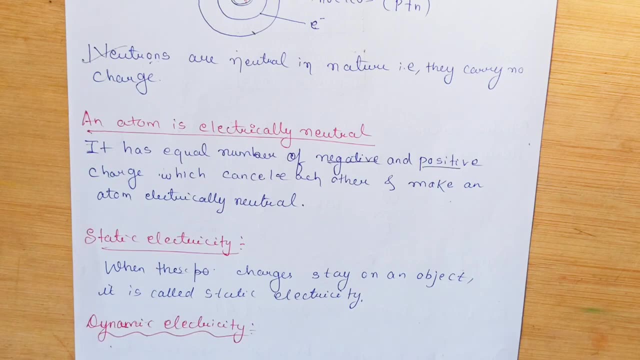 This atom is electrically neutral. After that, static electricity, Static electricity. So what is the meaning of static electricity? Let's see. Okay Now we just talked about the charge of electrons and protons. Normally what happens is that, if they are staying in an object, 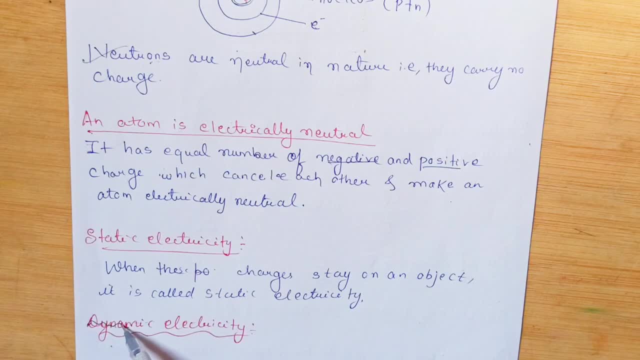 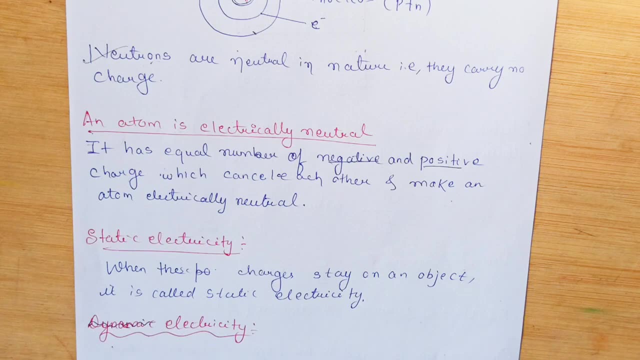 Okay. If they are staying in an object, then we will call that charge. static electricity Means the electricity that will come. there is called static electricity, But normally the current that we are observing at home, the electricity that we are getting. that happens basically because of moving charges. 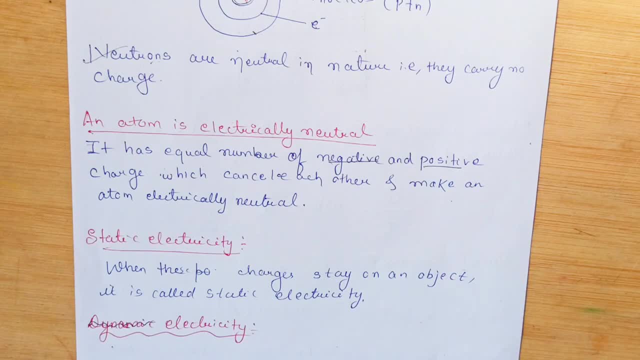 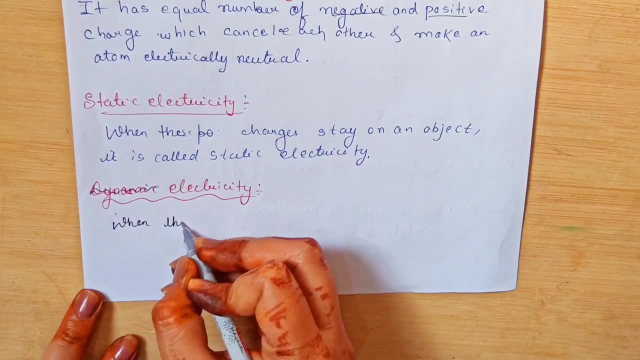 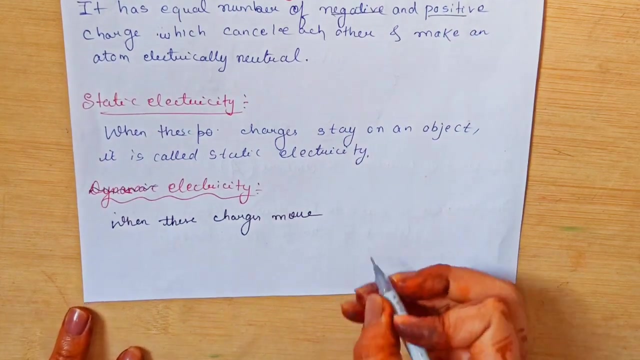 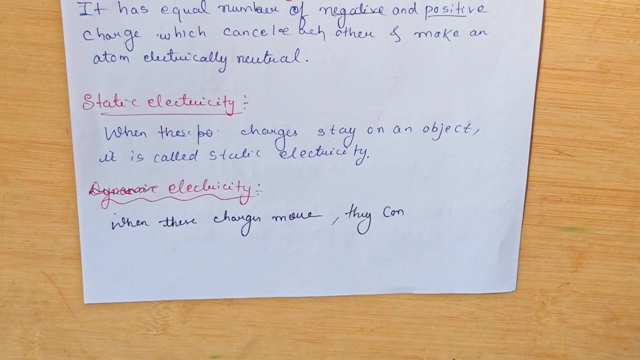 Here the charges stay in the object. But we don't need to know this. We need to know that, basically, when these charges move, when these charges move, then which electricity or which current comes because of them? We call that simply electric current or you can call that electricity. 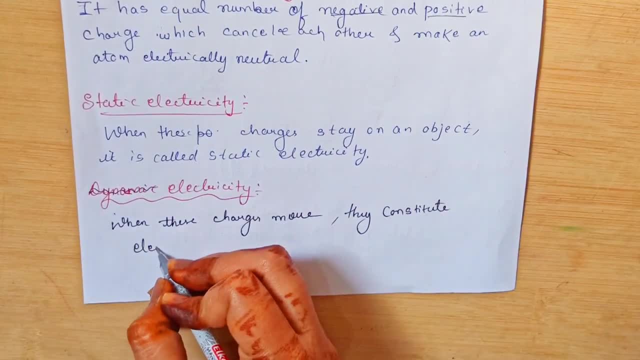 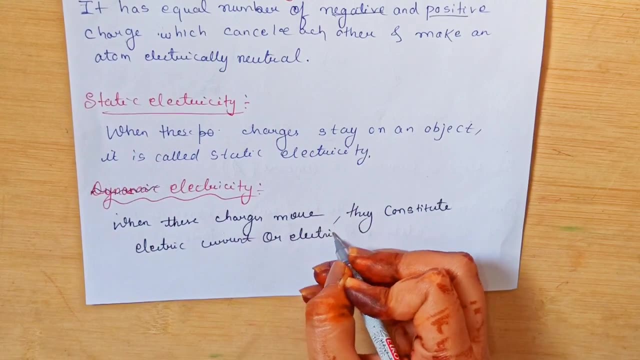 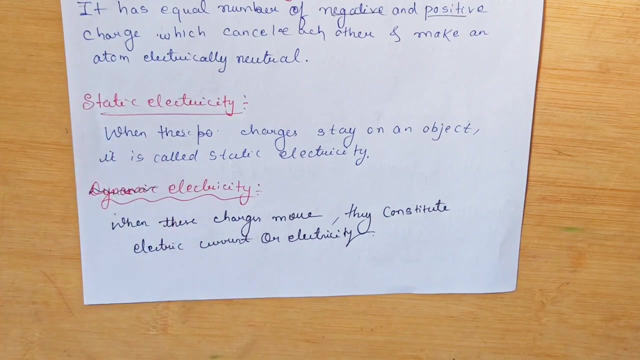 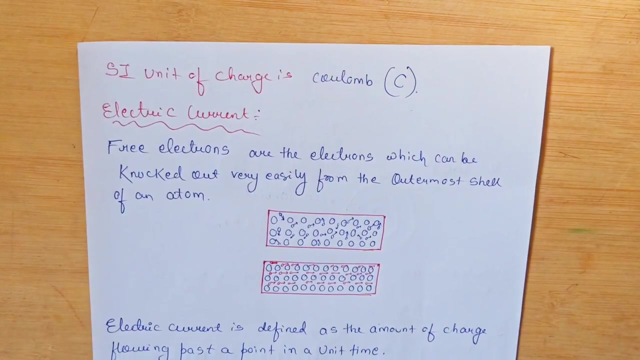 It depends Electric current or electricity, Okay, Okay, So normally one is static electricity and one is simple electricity. Okay, Now we will talk about this. We have studied so much about charge, So let's talk about its unit, About unit. 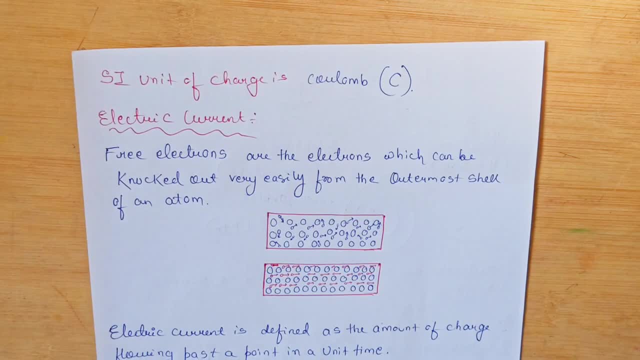 Like the mass, The weight. Its unit is kg, Isn't it? What is such a unit? It is kg, Kilogram. Similarly, the mass, The charge. Their SI unit is coulomb. What is coulomb? 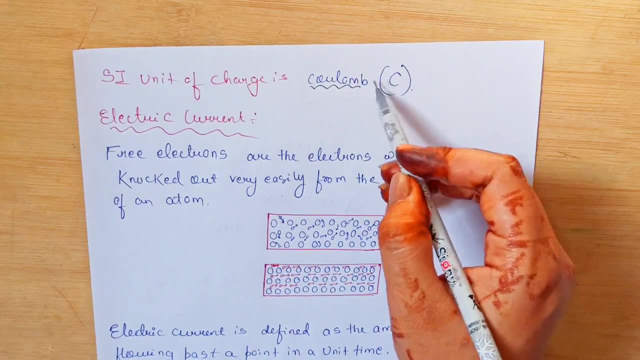 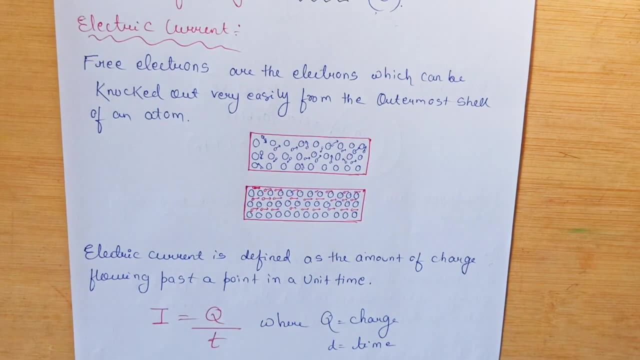 When you write it as symbol, write it as capital C, But when you are writing the name, write it as small c. Okay, It is important. Now how will we define electric current? We can't say like this: When this charge moves, that is called electric current. 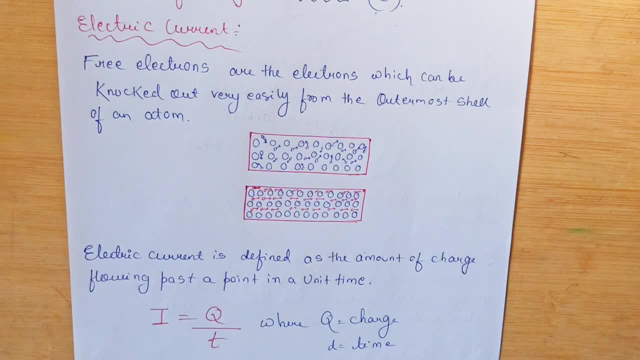 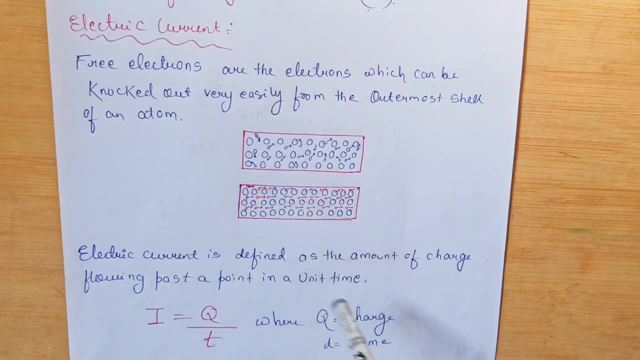 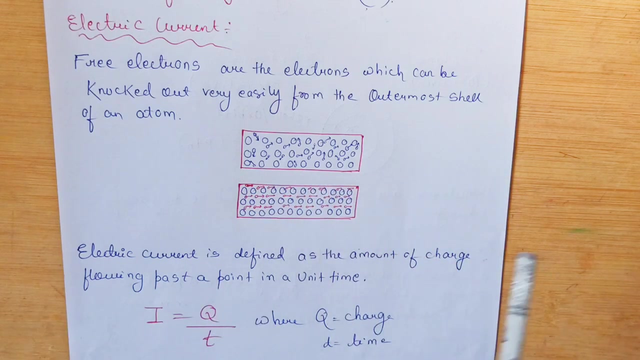 No, We can't say like this: Okay, We will talk a bit about electric current, Let's see what all is there. Okay, Suppose this is a substance. Okay, Suppose this is a substance. Now, we all know that the atoms in any substance have electrons. 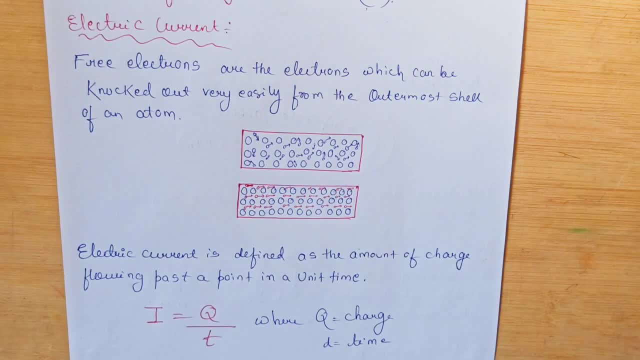 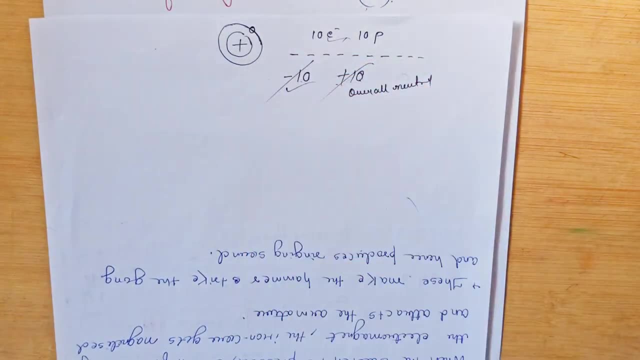 These electrons which are in the last shell Suppose. Here you can see the atom and this is the last shell of the atom. so we can easily take out the last shell of the atom. If they are free, then we will call them free electrons. Atoms of most metals contain very loosely bound, negatively charged electrons in their outermost orbit. 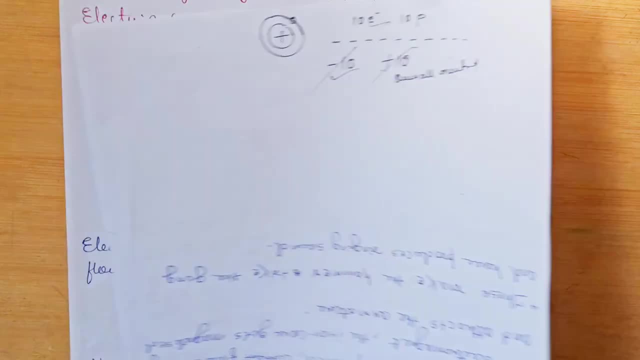 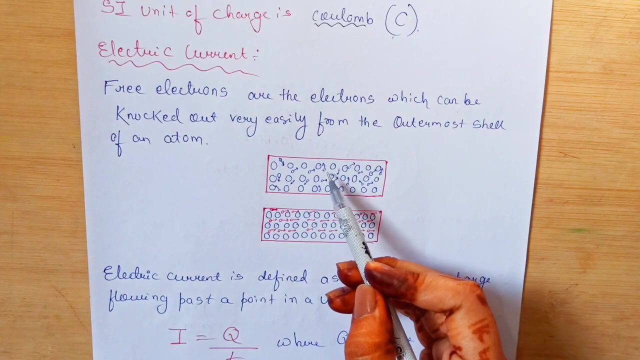 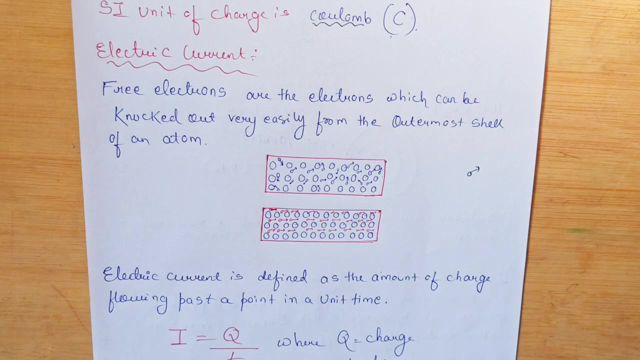 If we can take out these electrons, then we can call them free electrons. How can we define free electrons? You can see that these are free electrons. The electrons that I have made are free electrons. Free electrons are the electrons that we can take out from the outermost shell of the atom. 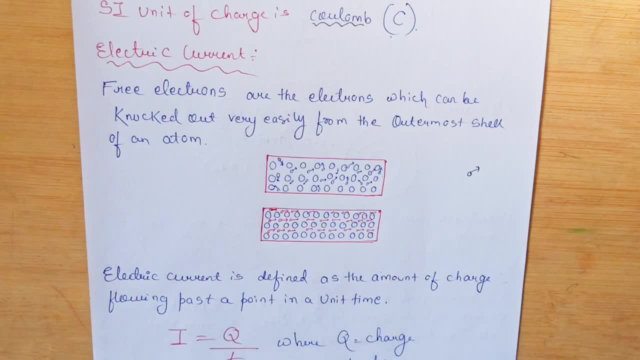 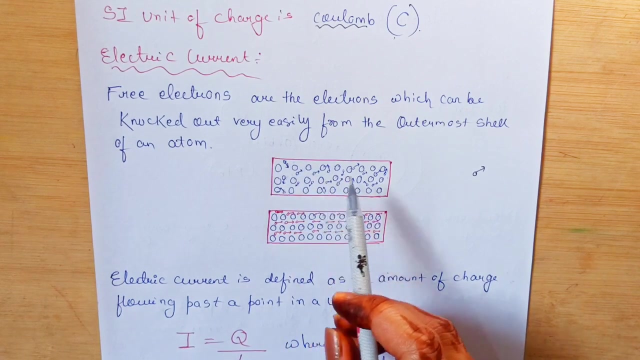 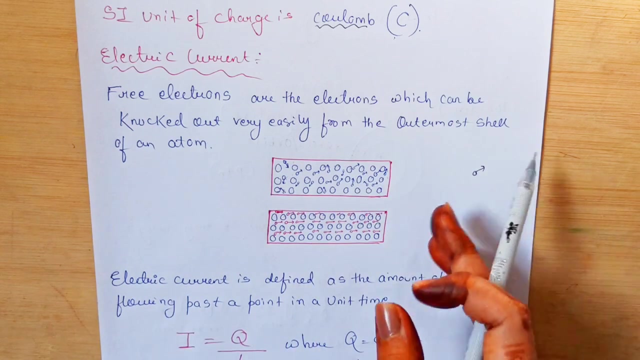 You should know that the electric current that we get to see is only because of the electrons. There is no role of protons there. In normal condition this is free electron. Here you can see free electrons. In normal condition they move randomly in all directions, But if we align them in a particular direction, 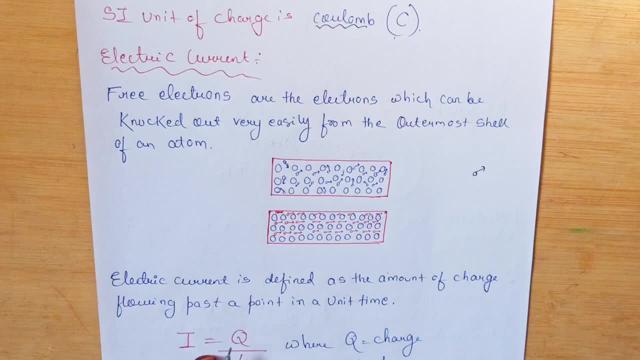 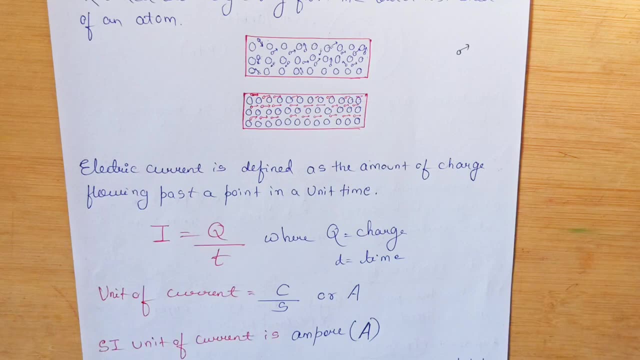 If we go in one direction, then we get to see the electric current. At that time we get to see the electric current. Now you are getting to see the electric current in my house. This means that the free electrons are moving in the same direction. No one is doing it on their own will. 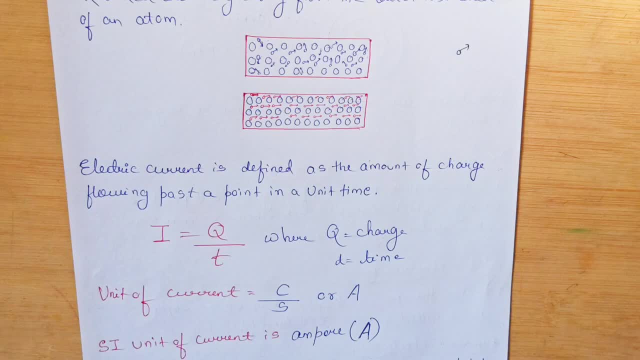 They are all moving in the same direction. How can we define the electric current? The electric current is the amount of charge flowing past a point in a unit time. Suppose here, From one place In one second, How much charge went away? That is called electric current. 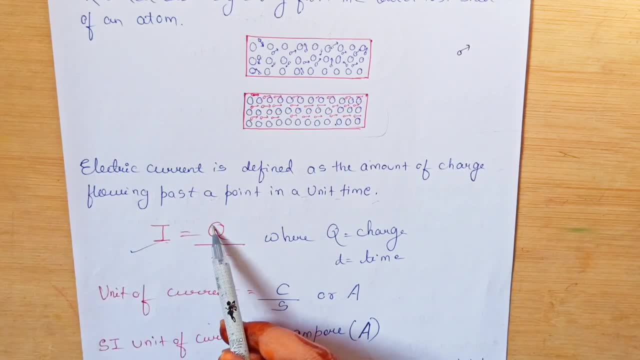 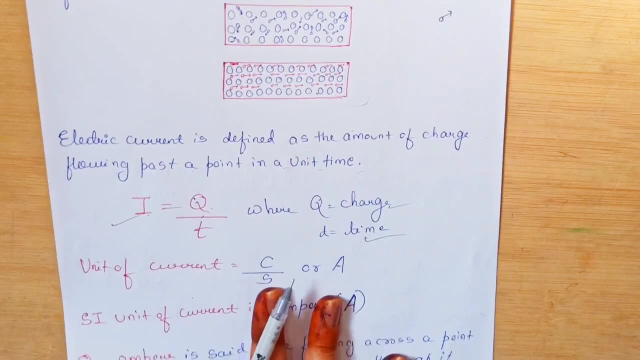 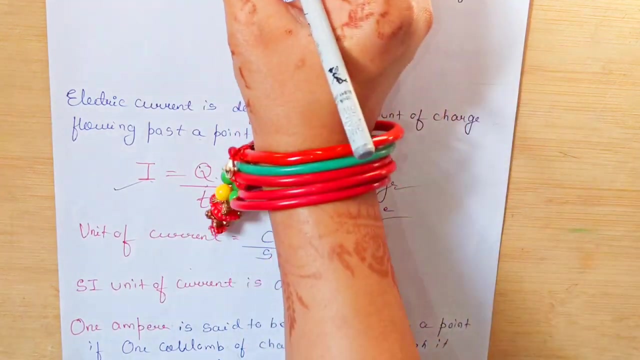 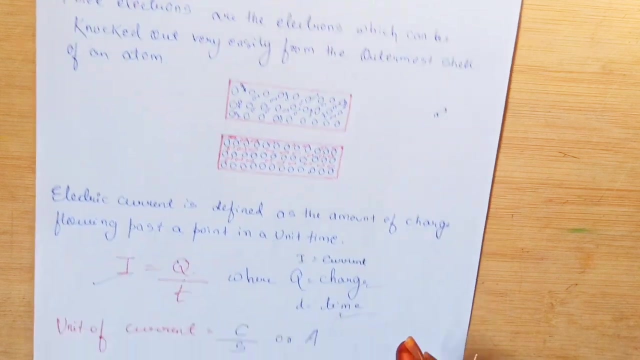 We write I for electric current, We write Q for charge And we write T for time. Sorry, we write T, So here T is the time, Q is the charge, I is the current. I is the current. I is the current. Okay, Here I is the current. The symbol of I is used for current. 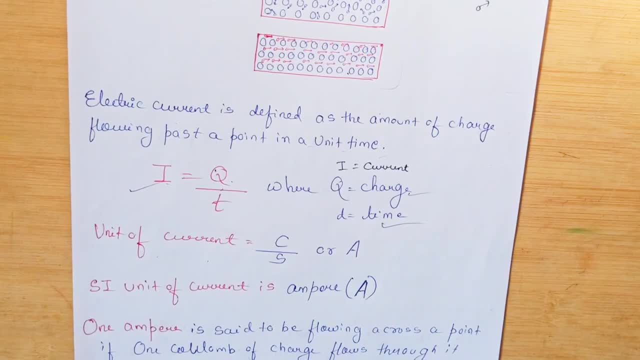 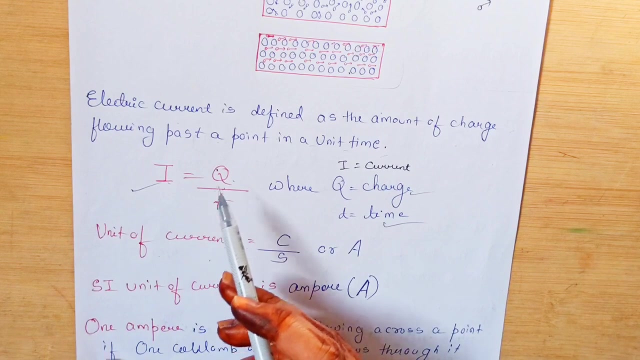 Don't write I Okay. So how can we define the electric current? How much charge is flowing from a point in a second? How many free electrons are coming out? That is called electric current. So how can we express it mathematically? I is equal to Q by T.